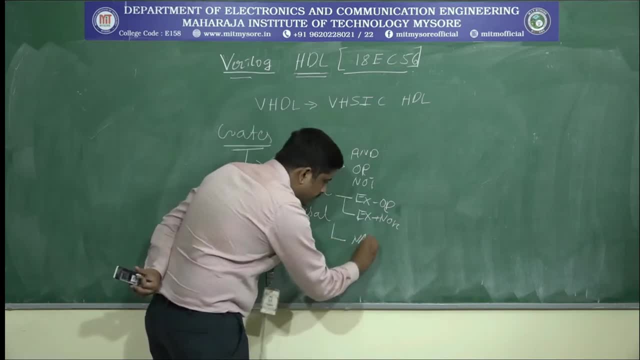 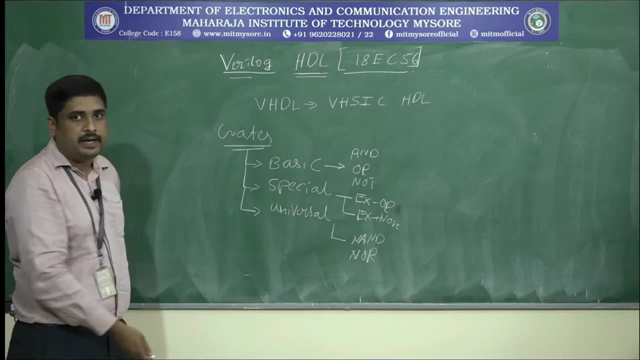 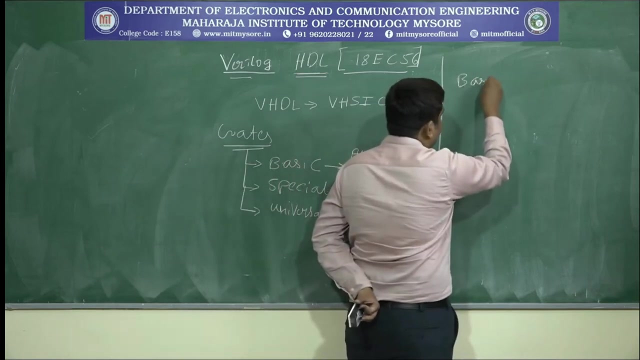 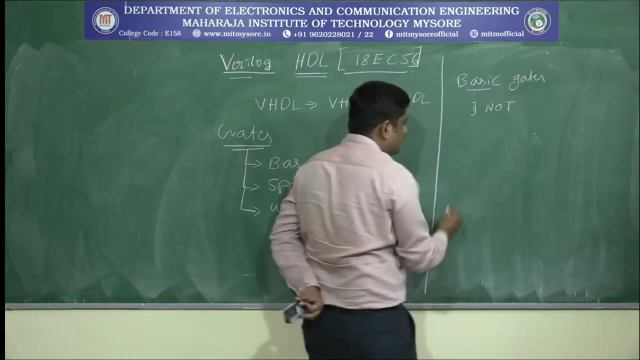 There are two universal gates. one is NAND, another one is NOR gate. We need to know all these gates in detail. So first we consider basic gates, First one NOT gate. First we write the symbol of NOT gate. This is a symbol of NOT gate. 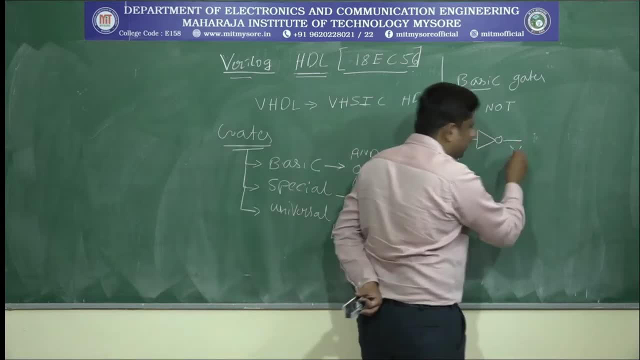 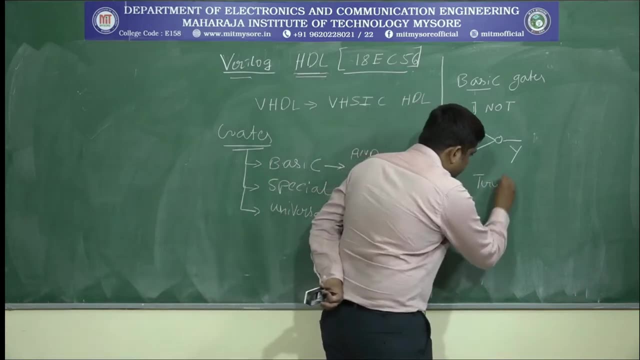 Let us assume one input then as well as one output. So once you mention the input and output, next we write the logic That is using truth table. So once you mention the input and output, next we write the logic That is using truth table. 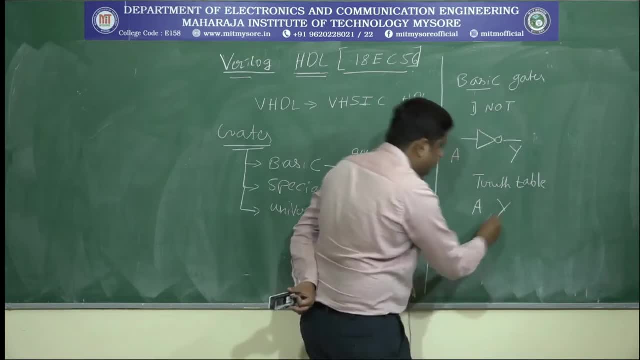 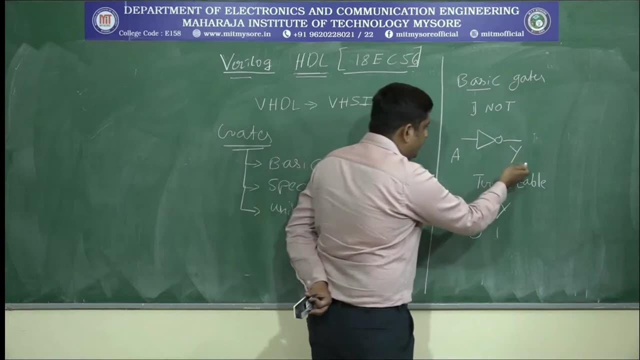 table. then a is the input, y is the output, then a is equal to 0, then y is equal to 1.. When you applied a is equal to 0, then we getting output side y is equal to 1.. Then you applied a is equal. 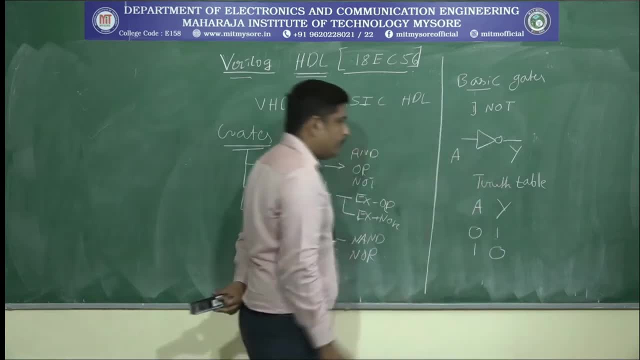 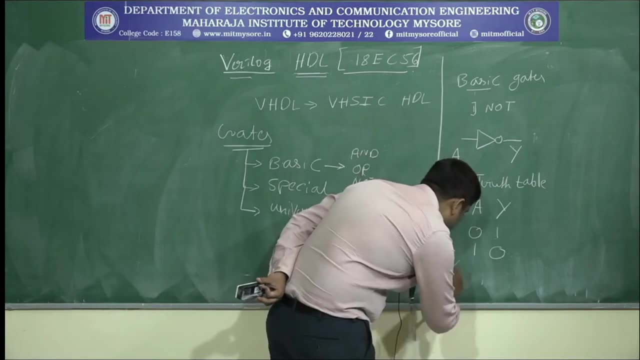 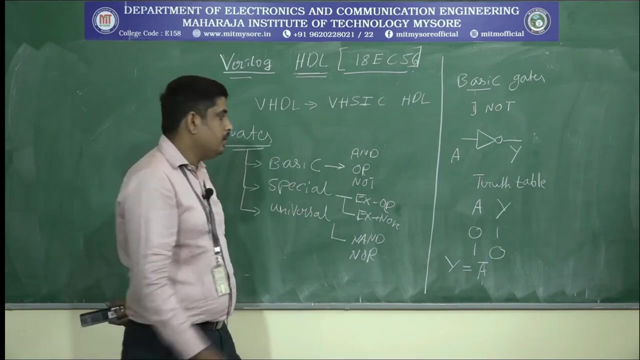 to 1, then we getting y is equal to 0.. So, based on this true table, we have to write the equation. So the equation can be written as y is equal to a complement, or we called as y is equal to a bar. So here, based on this equation, using this equation, we have to write the programming that 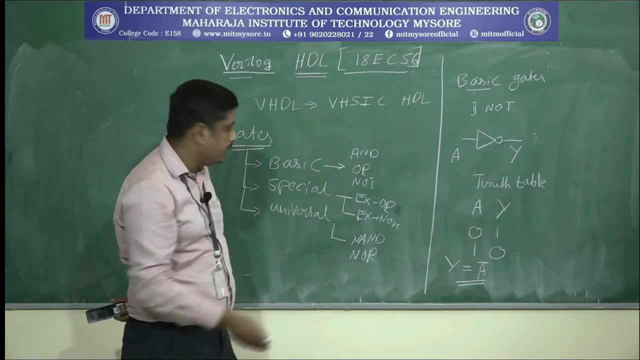 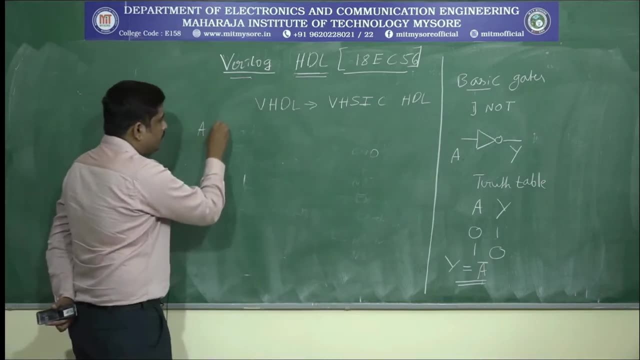 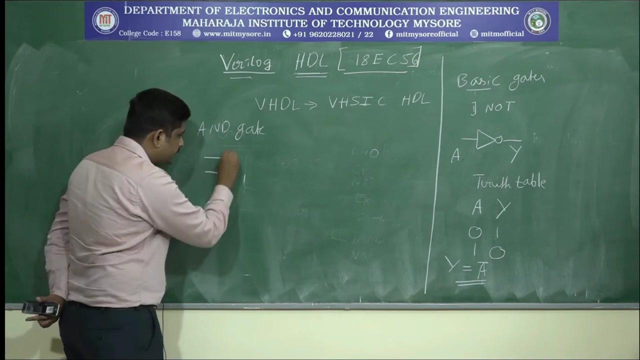 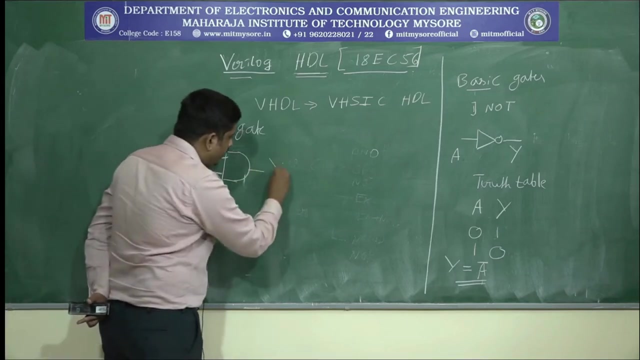 is Verilog code later. First we studied this, not gate, then next move on to second one, And gate. first again we write the symbol of and gate. So there are two inputs here we assume a and b, then one output it is again we consider it is y, then next we write the true table for this gate. 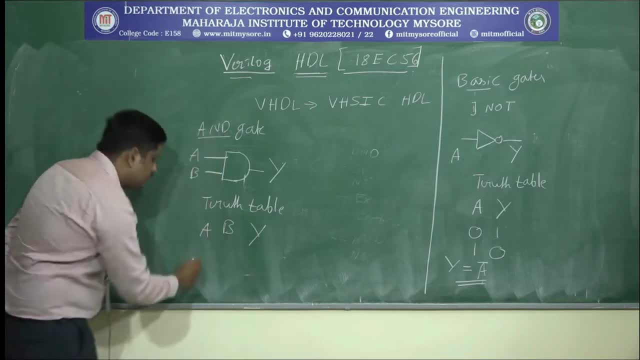 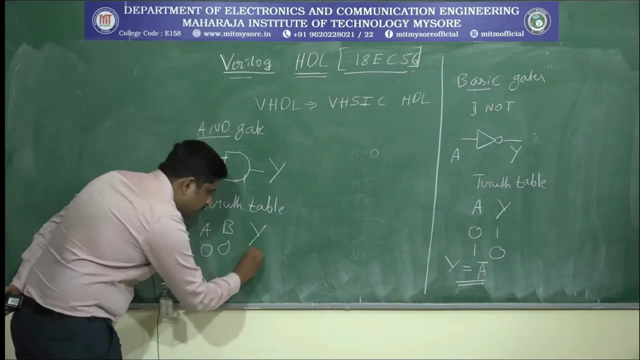 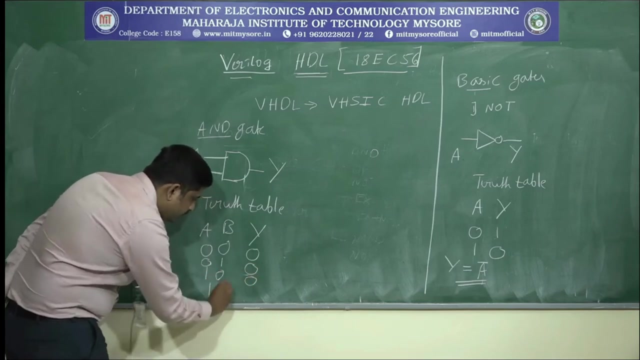 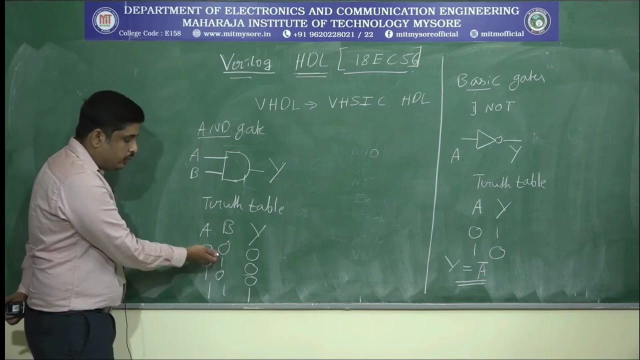 Here the name indicates and gate. So first assume 0. Here there are four combinations here: first 0, 0, then output is 0, then 0, 1, output is 0, then 1, 0, then output is 0, then 1, 1, then finally getting output is 1.. So here any one of the input is 0. 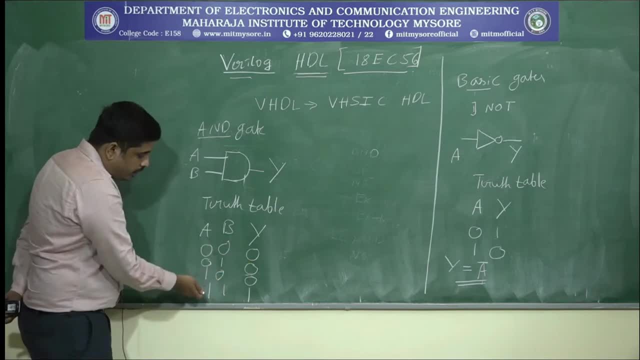 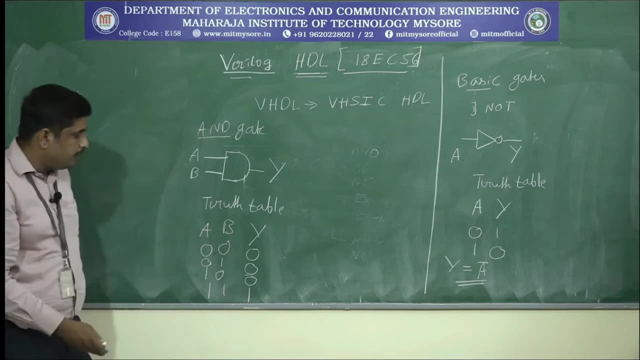 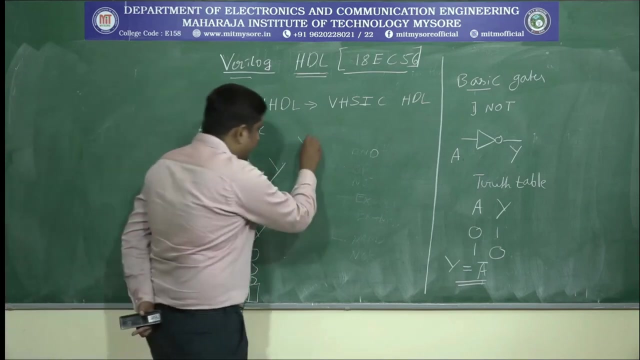 and that time output is equal to 0.. Then only one condition: all the inputs are i, and that time only the output is equal to 1.. So after this true table We just mark the what when the output is equal to 1, then write the equation here: y is equal to a and. 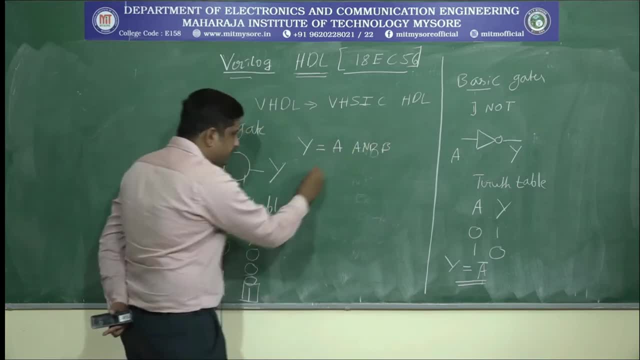 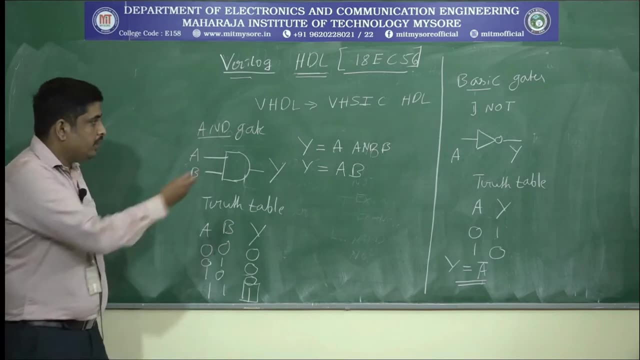 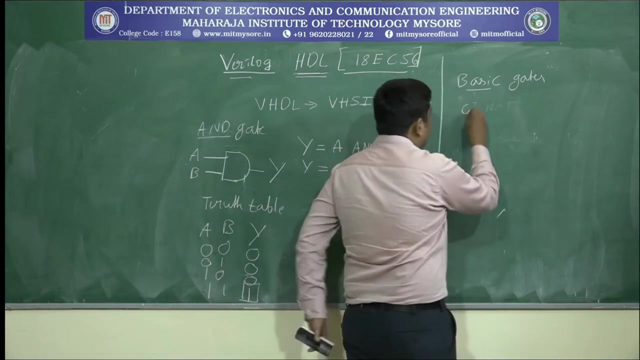 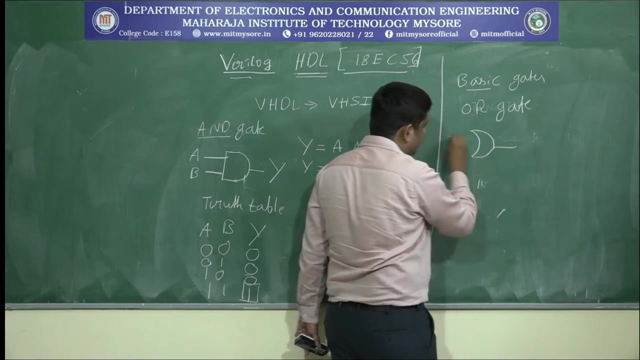 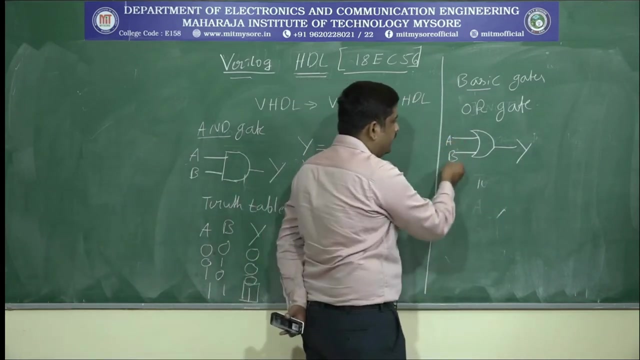 b, or we simply write y is equal to a b or a dot b, like this. So here getting the equation that is y is equal to a b. then we can possible to write the Verilog code for this one. Next third one, or gate. this is the symbol of, or gate. two inputs: a and b, then y, then write the true table. 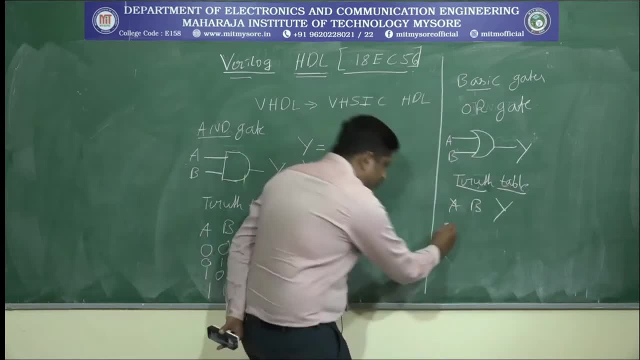 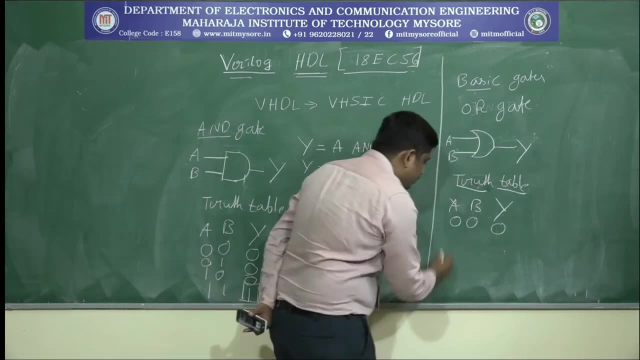 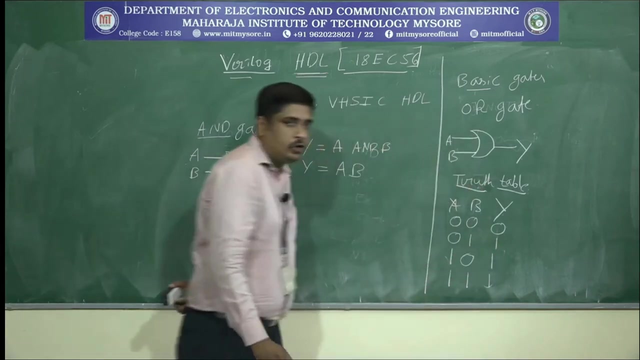 Again here four combinations. it's similar to and gates. So first combination: if it is 0, 0, then output is 0. if it is 0, 1 output is 1, then 1, 0 output is 1, then 1, 1, 1. the output is equal to 1.. Speciality: 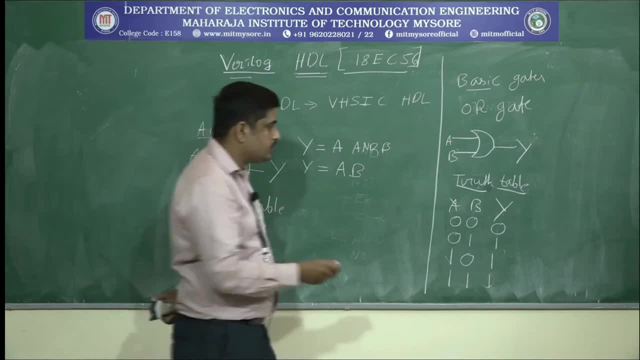 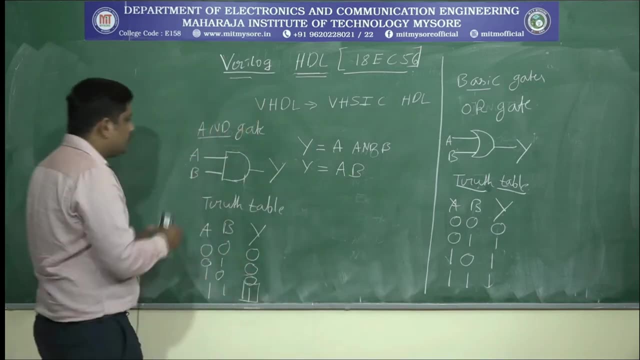 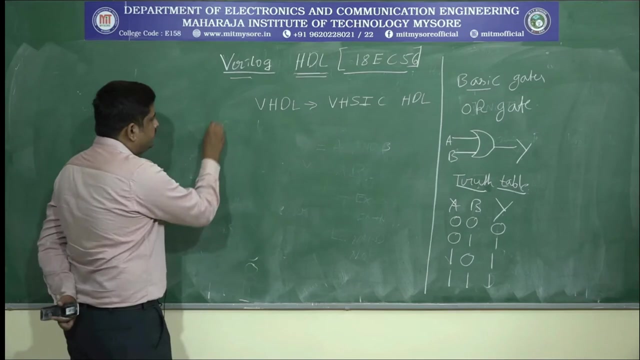 of or gate. here the any one of the input is high and that time output is equal to 1.. This is the what a or gate. Next move on to Special gates. The first special gate we have to consider XOR gate. This is the logic symbol. then a and b is the input, then y is the output. Next we write the true table. 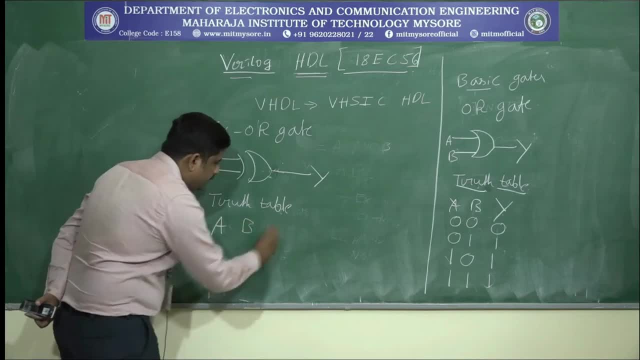 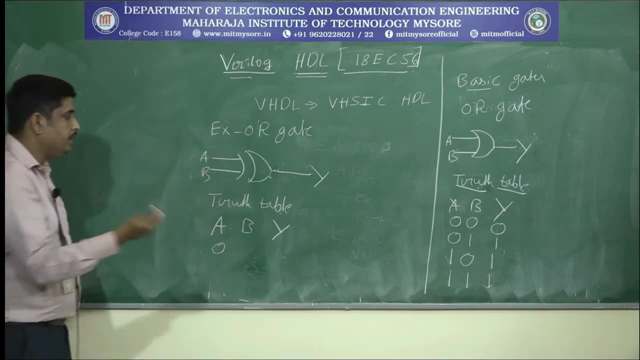 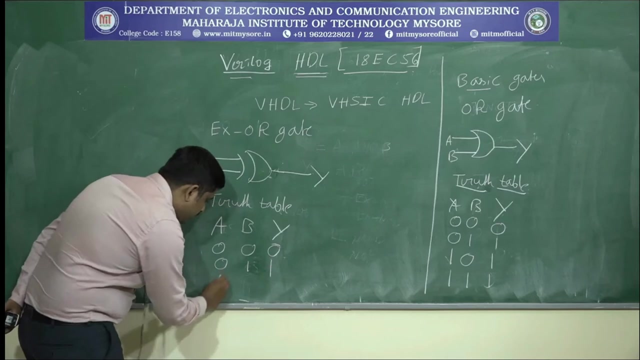 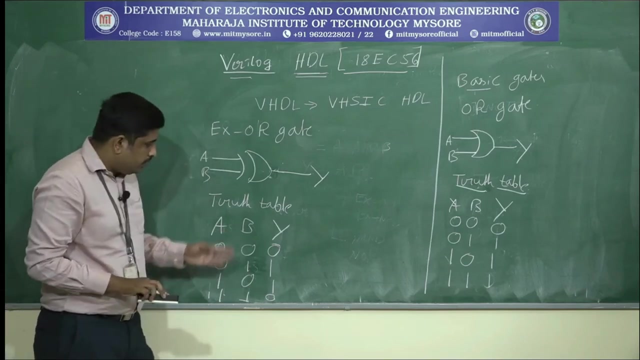 So here we have a and b, then y, then first again similar to what previous gates, that is R, and there are four combination here: 0, 0, then if it is 0, 0, 1 it is 1, then 1, 0, 1, then 1, 1 it's 0.. Just observe the true table here. Why we called as special gates? because here the condition when. 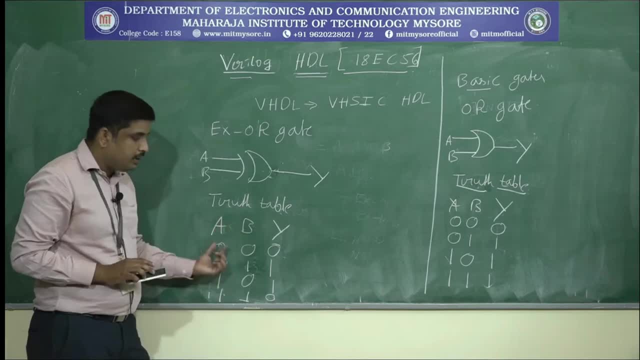 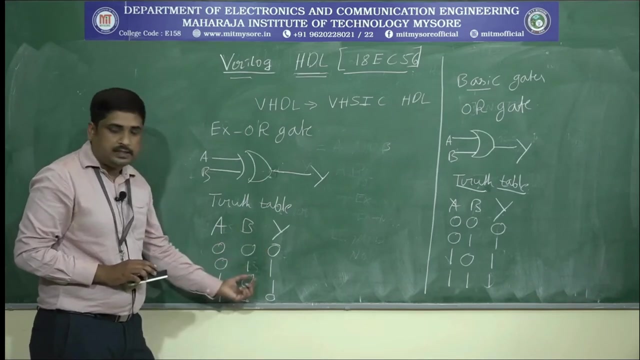 all the inputs are either low or high, all the inputs, and that time only it's logic 0.. If any one of the input is complement, for example a is equal to 0, then b is equal to 1.. Suppose a is equal to 1, b is equal to 0, and that time only the output is what Logic 1.. So 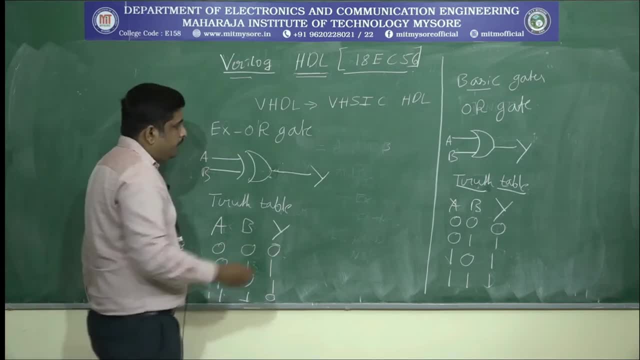 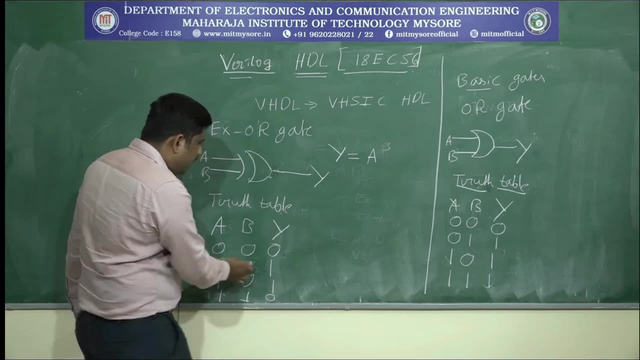 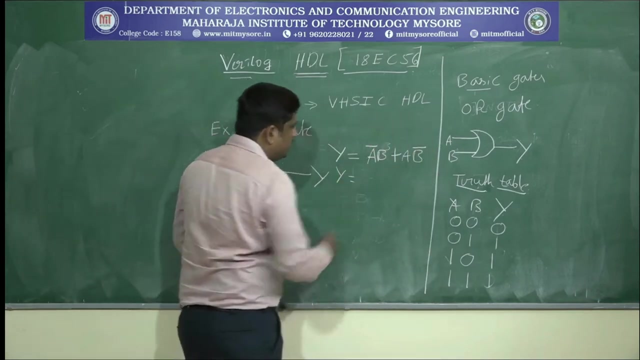 based on this output, we write the equation that is y is equal to here: first one a bar b, that is a complement b plus. then this is the what R gate, then next one a bar b, then a b bar. So here, just observe the equation. So compared to previous equations it's little bit complicated. 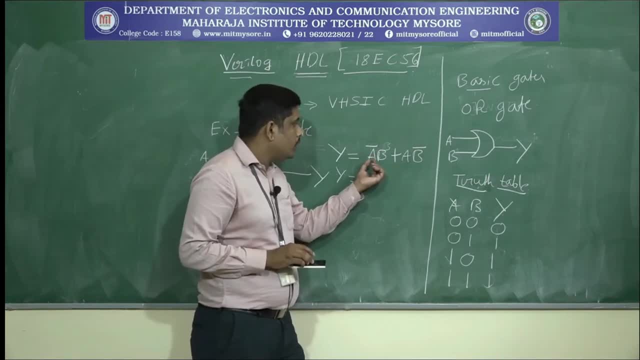 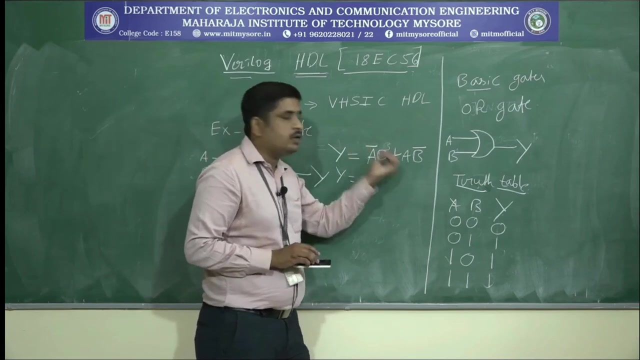 because here, when you complement the, what a one, not gate is required. When you complement the b, one more not gate. So two, not gates is required. here then plus two and gates: a bar b one and gate, then a b bar another and gate, then totally four plus one. 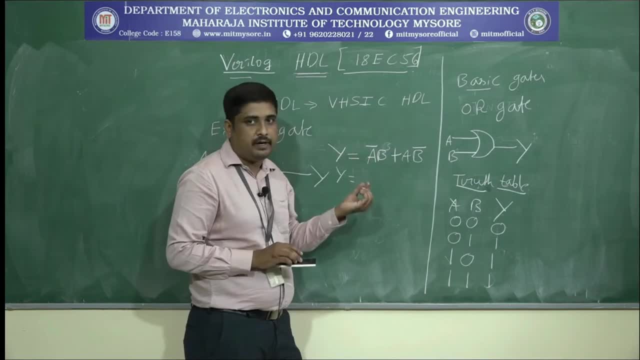 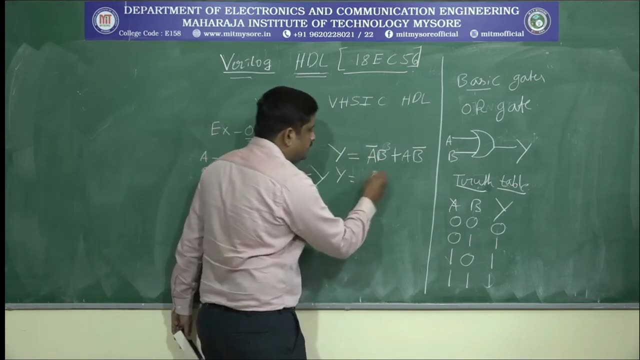 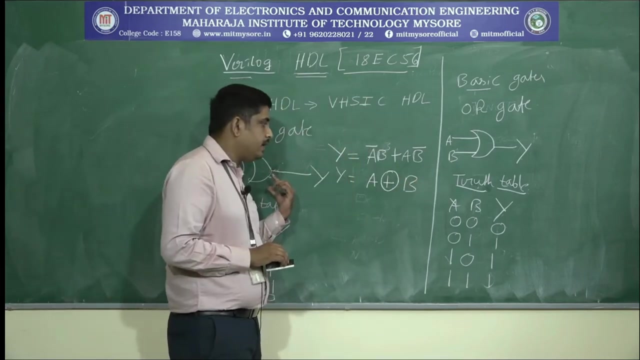 R gate. So totally here. there five gates are required. So it's very complicated. That's why we write the. we just modified this equation. that is a exclusive or b, So there is a. what Special XOR gate is there? We can directly write: y is equal to a exclusive. 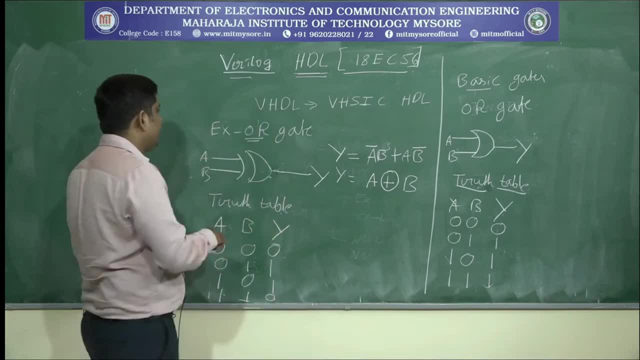 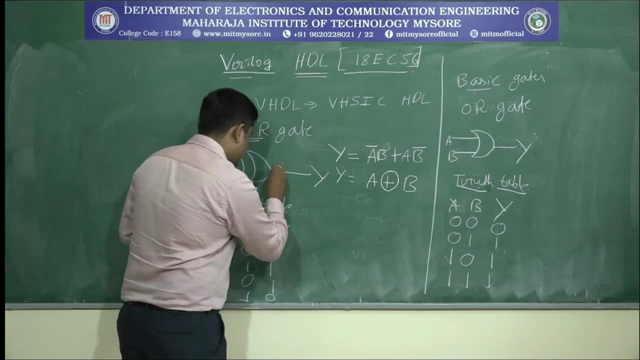 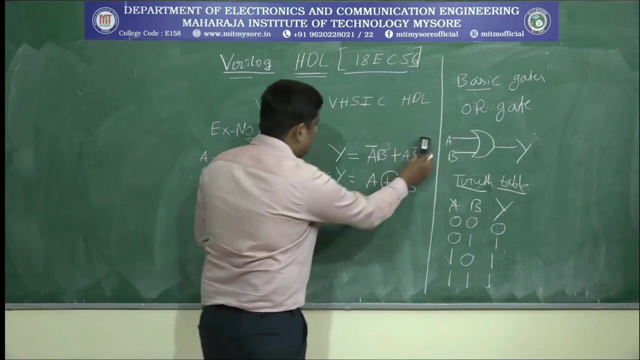 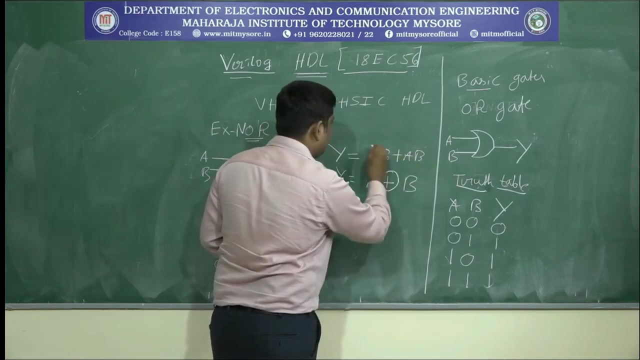 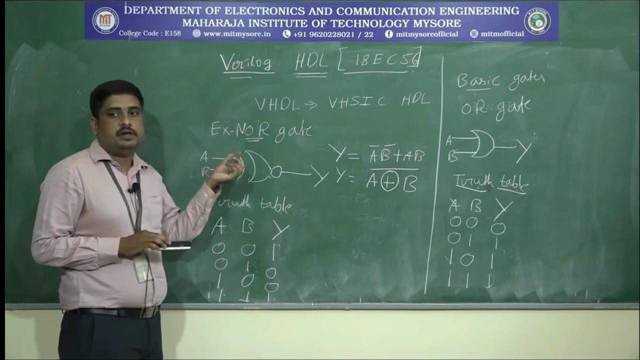 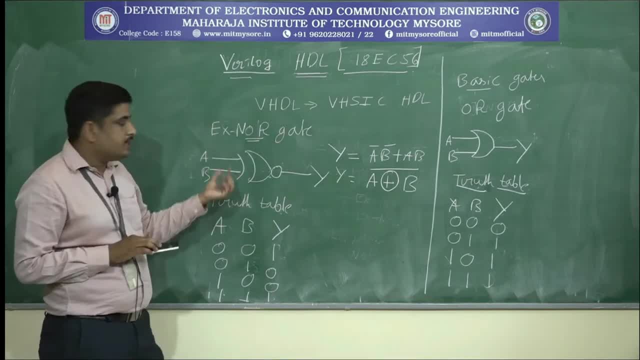 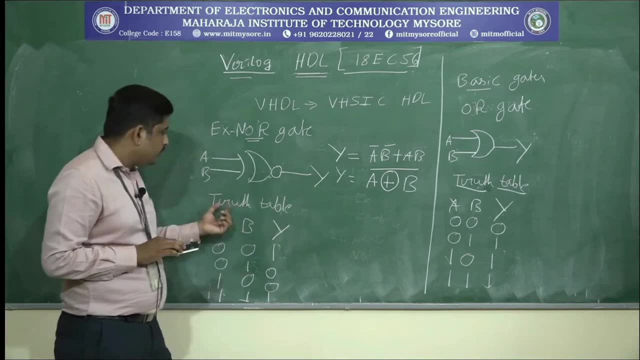 here we called as XNOR gate, So this is the symbol of XNOR gate. then a and b is the input, then y is the output. then truth table: a, b, y. when it is 0, 0,, then it's 1,, when it is 0, 1,. 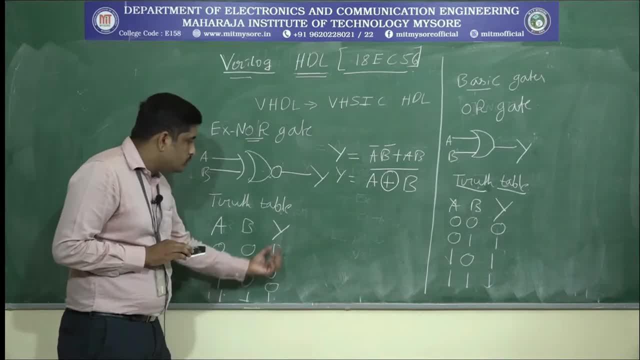 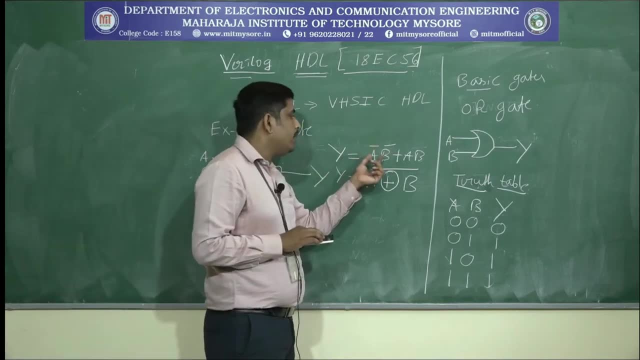 it's 0,, 1,, 0, it's 0,, then 1, 1, it's 1.. So it's exactly opposite of what The the same, the previous one, XOR gate. So here, this is the equation: y is equal to a bar, b bar plus a b. 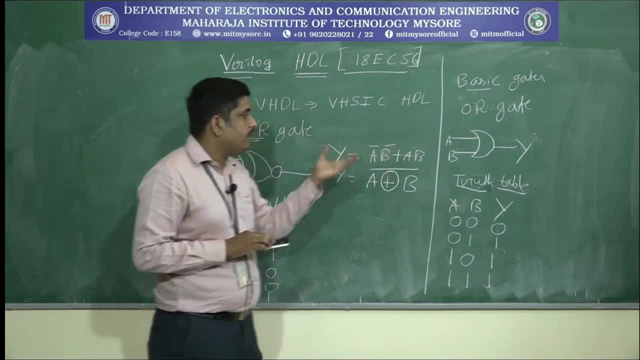 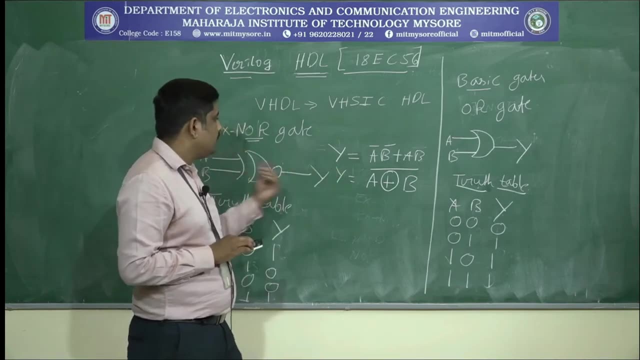 So using this equation- it's very difficult one. Again- it requires totally five basic gates. So that can be modified using in terms of: we write: XNOR y is equal to a, XNOR b, that is a XNOR b. 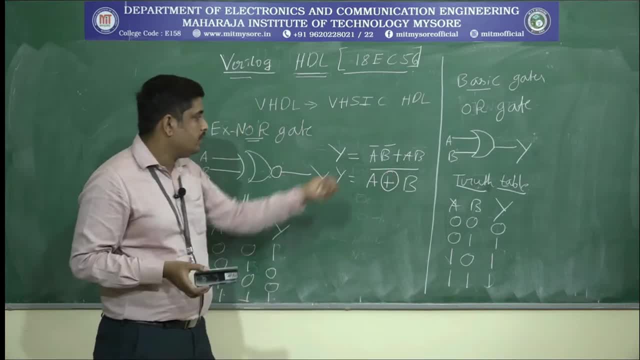 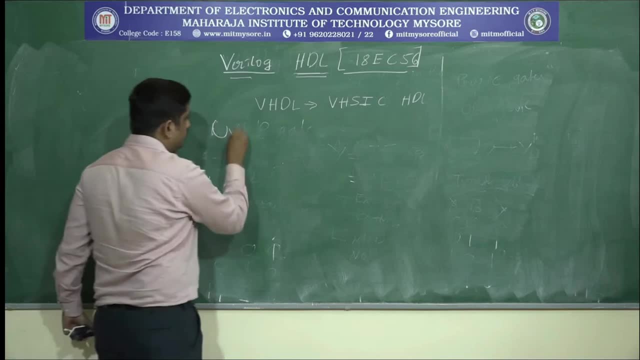 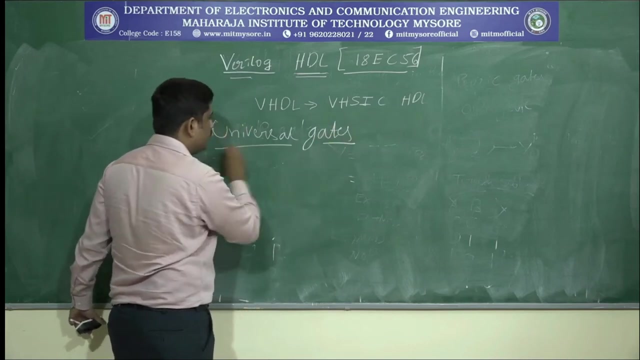 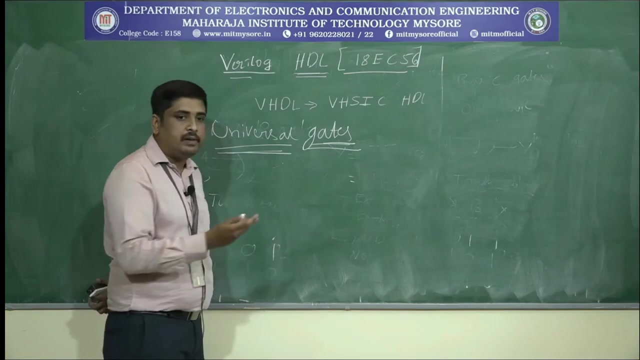 So using this equation we can possible to write the program torane for this equation. Last type of of gates, So very important one: universal gates. So first the definition why we called as universal gates? Because using this universal gates we can possible to design any gate. 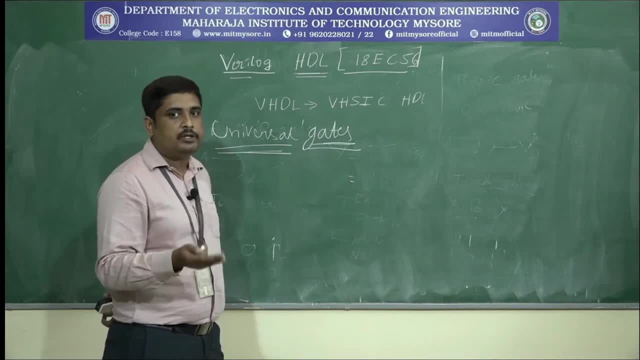 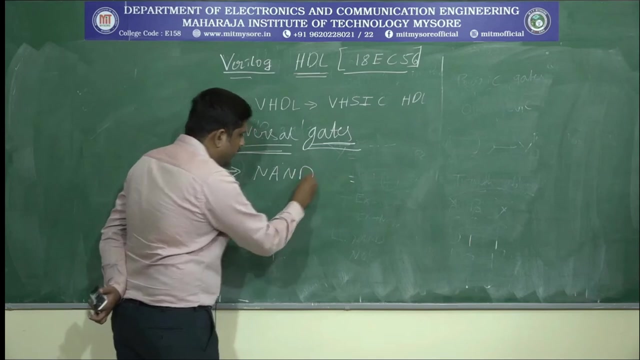 we can possible to design AND gate. we can possible to design OR gate and also NOT gate. and also we can possible to design a special gates using universal gates. So universal gates, two universal gates, one is NAND, another one is NOR gate. So first we consider: 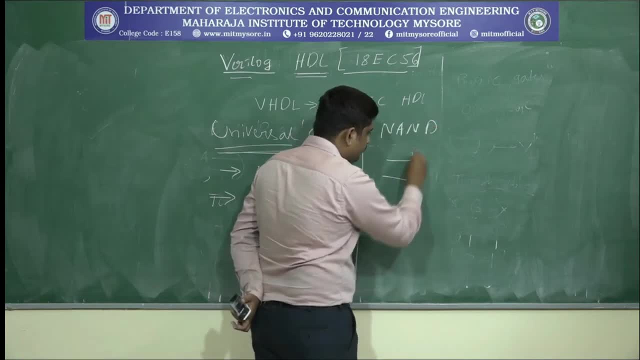 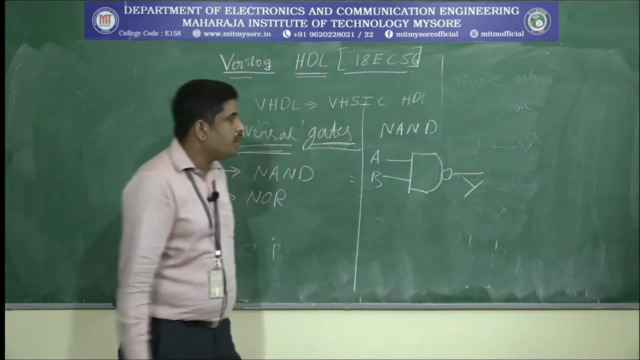 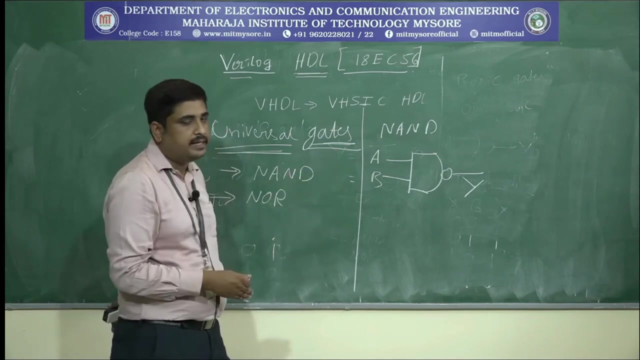 NAND gate. This is the what, A symbol of NAND gate. So it is exactly opposite of what AND gates. You just consider AND gate. we just add one inverter or NOT gate at the output side, then it becomes an NAND gate. So here we directly write NAND gate symbol. here, Then after this: 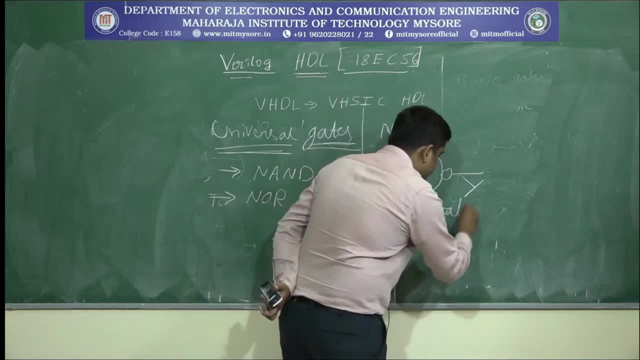 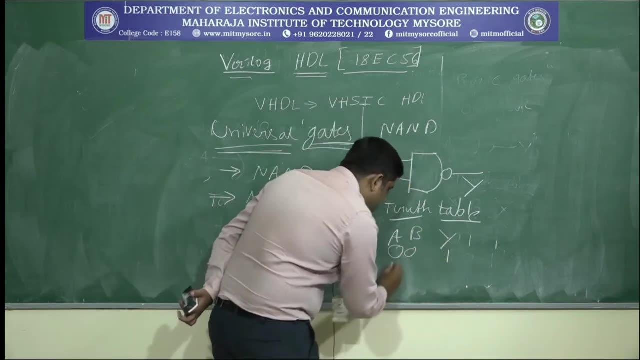 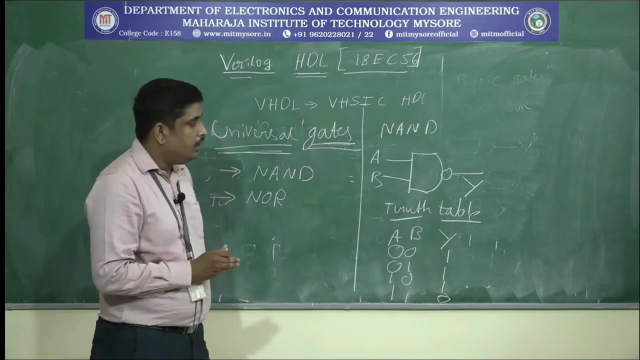 true table, then A and B is the input, Y is the output. So if it is 0: 0, it is 1, 0, 1, 1, 1 0, 1, 1, 1 0.. After this true table it is exactly opposite of AND gate. All the inputs are I and that. 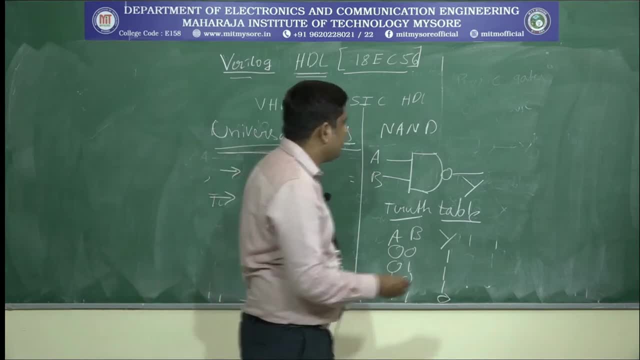 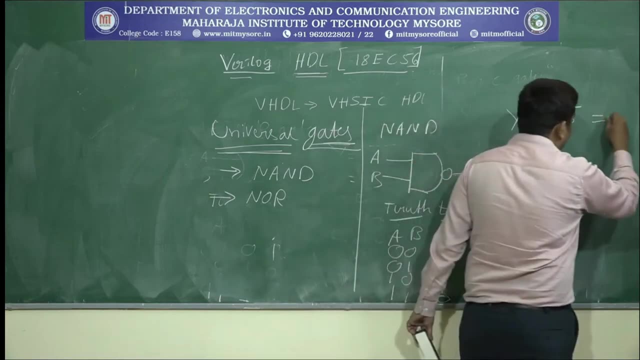 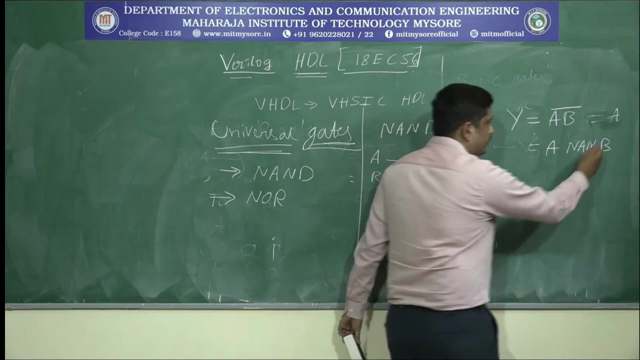 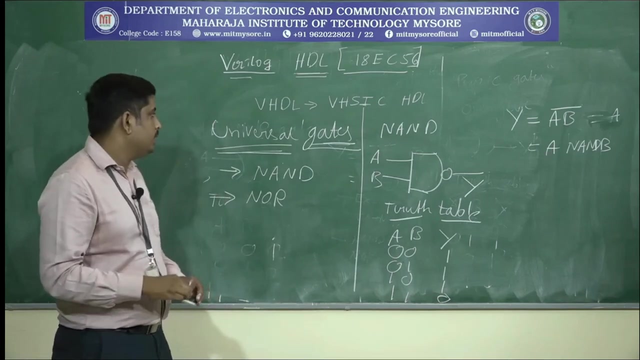 time the logic 0.. So after this we write the equation for this NAND gate: Y is equal to A B complement. or we can write: is equal to 0.. A NAND A NAND B. So this is the what some explanation about NAND gate. 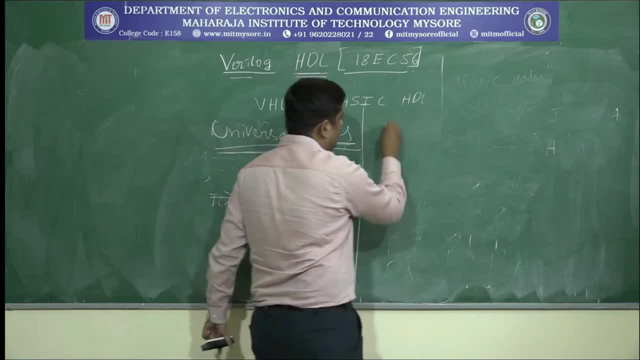 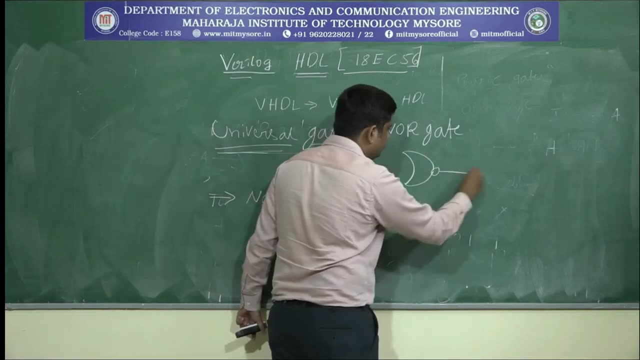 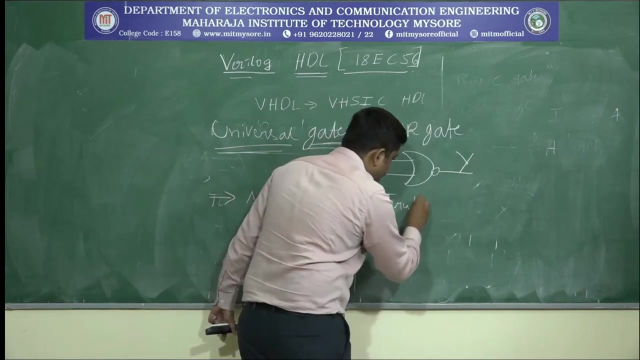 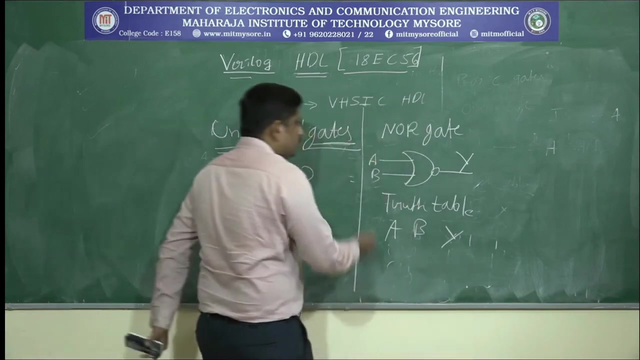 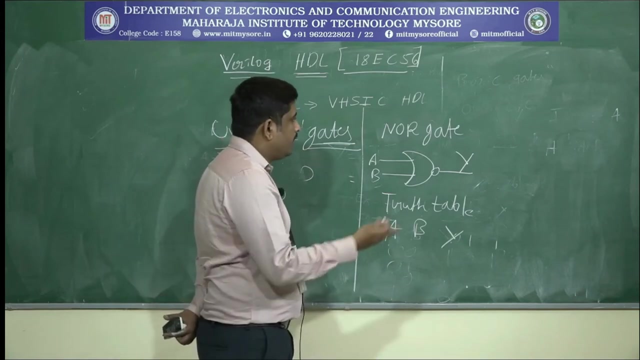 Next move on to next one: NOR gate. So this is the symbol of a simple NOR gate. So it's exactly opposite of this basic gate. So here we can possible to write one OR gate. it's just connected to serial with a NOT gate. 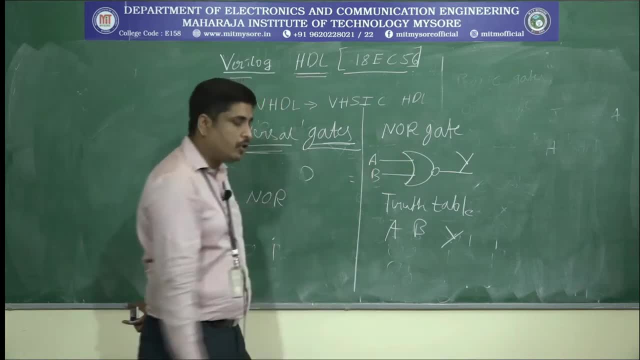 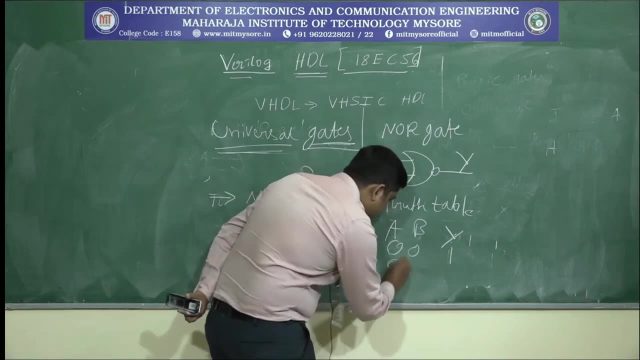 Then it becomes a NOR gate. So here this is a symbol of NOR gate. Then true table A and B: 0, 0, and that time it's 1.. Then 0: 1.. It's 0.. Then 1, 0.. 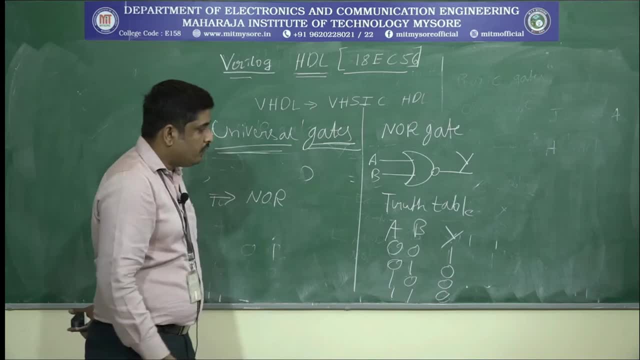 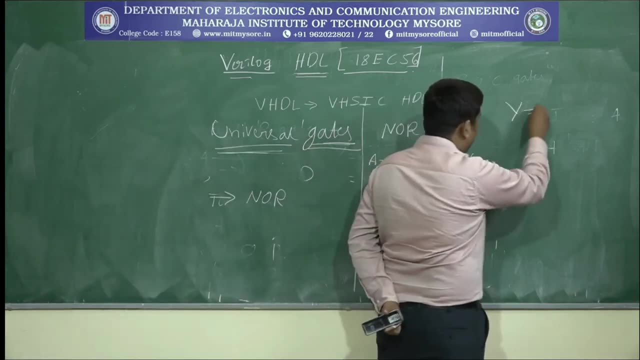 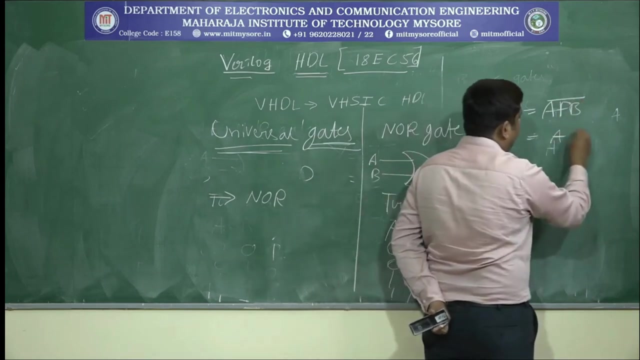 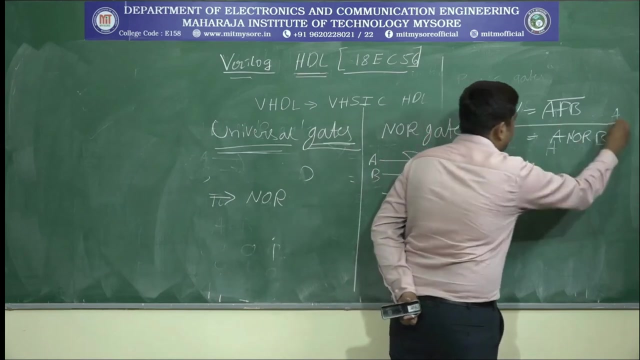 It's 0. Then 1: 1. It's 0. So it indicates when all the inputs are low and that time only the output is logic 1.. We write the equation here: Then Y is equal to A plus B, whole bar. or we write: A NOR B is the final equation for the 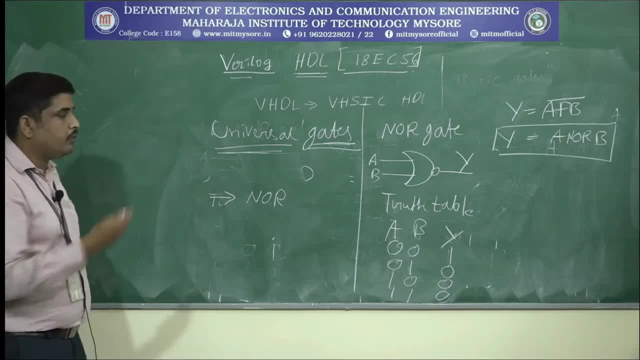 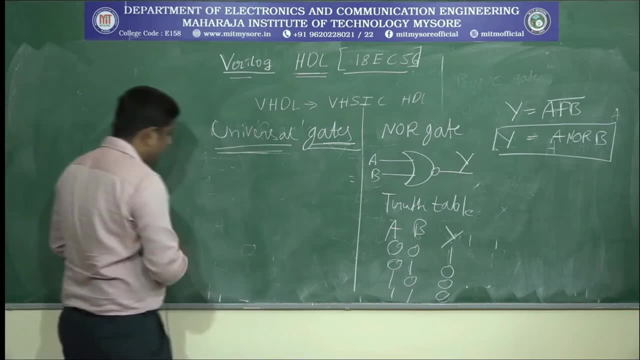 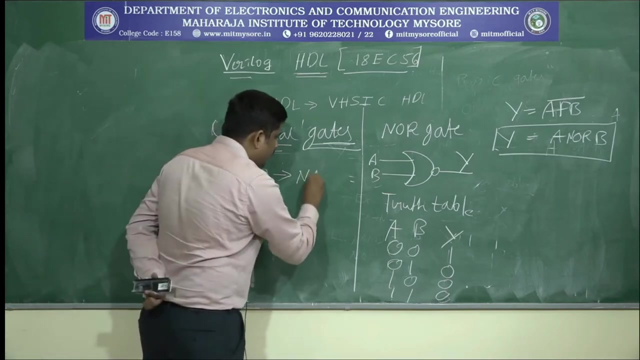 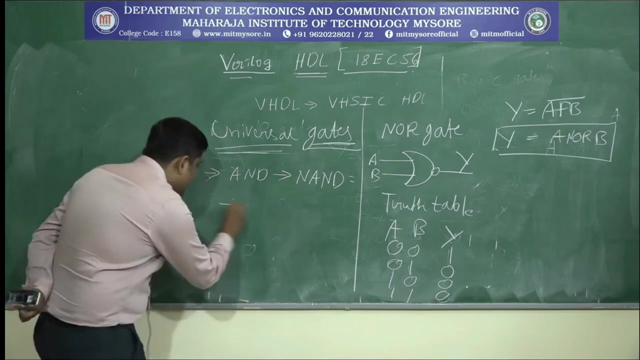 NOR gate. We divide it, We define It's an universal gate. We just prove it. the what the NAND gate or NOR gate, It's just an universal gate. So first we consider: we design AND gate using NAND gate. Design AND gate using NAND gate. 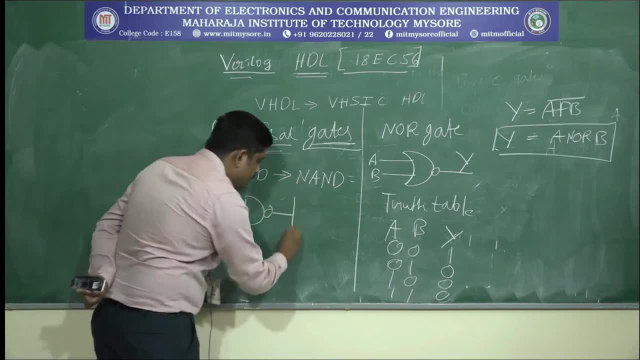 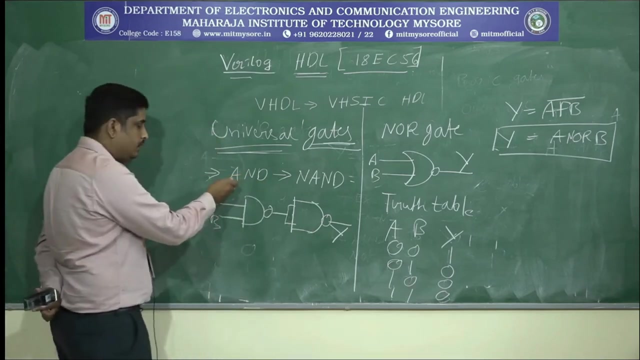 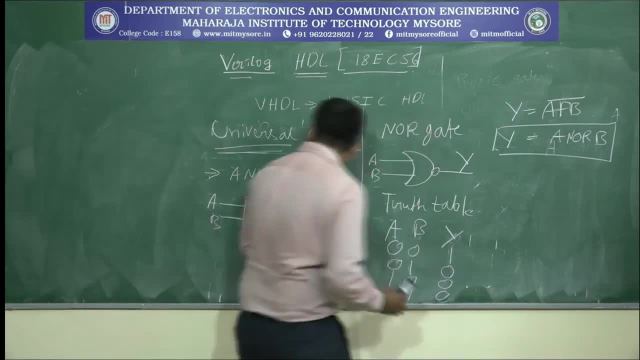 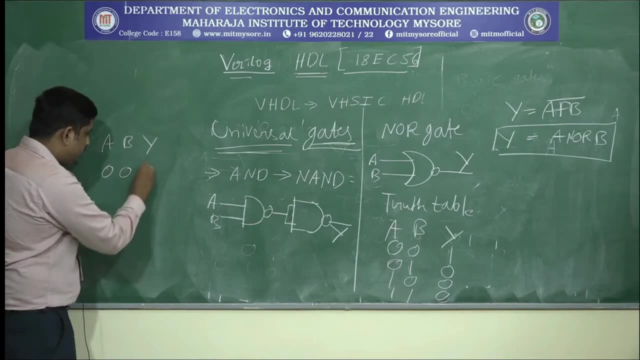 This is the what final circuit for AND gate using NAND gate. We just verify this circuit. Write the true table for the. Write the true table for AND gate here: 0, 0, 1, 0, 1, 0, 0, 1, 1, 1.. We just verified the year when you applied 0, 0 and that time. 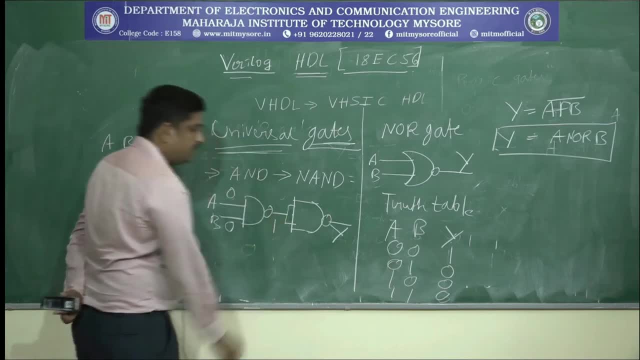 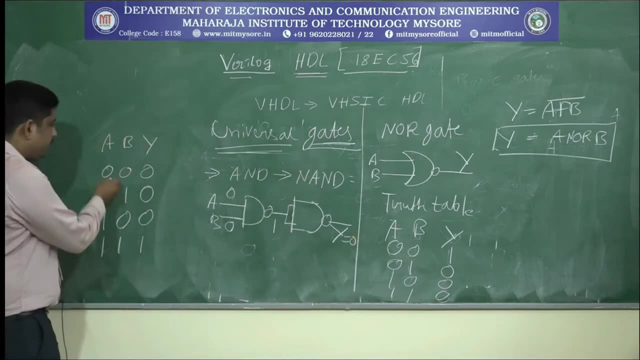 So we know that NAND gate root table: when it is 0, 0, then it becomes an 1.. When you applied 1, 1 year, then it becomes an 0. So when you applied 0, 0, then it becomes an 0 year. Next, take one. 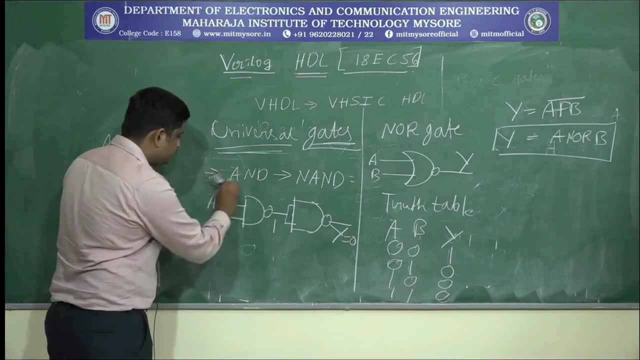 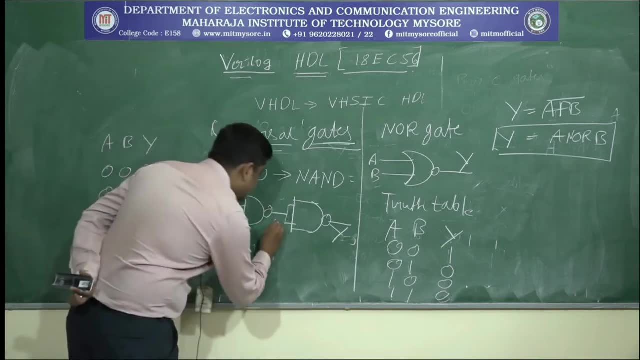 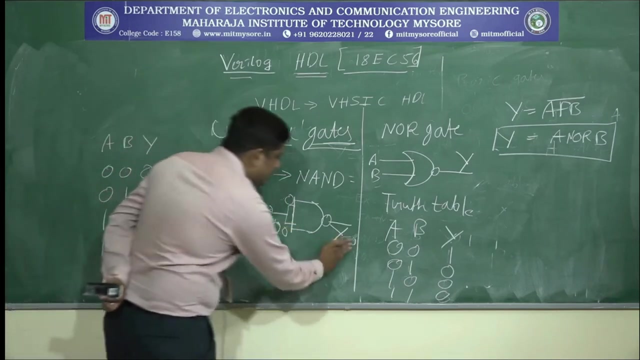 more reading. that is 1, 1.. When you applied 1, 1, then output is equal to 0.. At the NAND gate again here, 0, 0. then when you applied 0, 0, then output is equal to 1.. This is the what. 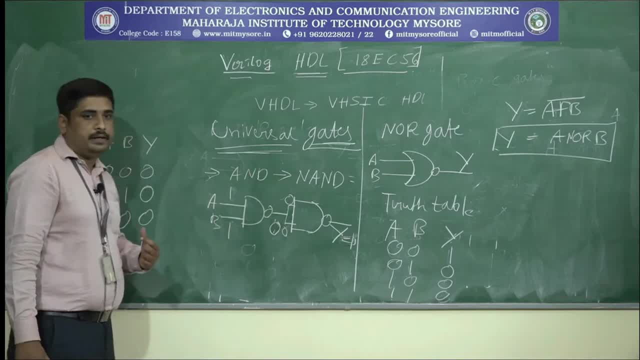 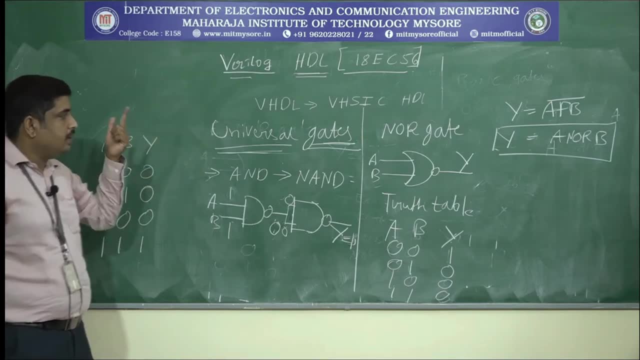 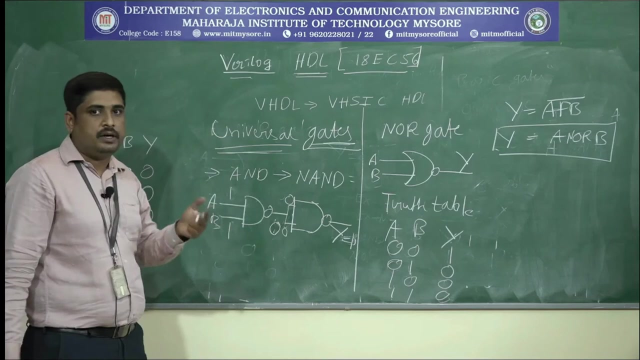 a AND gate circuit using NAND gate. Next here, these are all the what gates we have to studied, basically Basic gates, then special gates and universal gates. Next move on to a we have to design. next a digital circuits, digital system design. So here, generally two types of digital system. 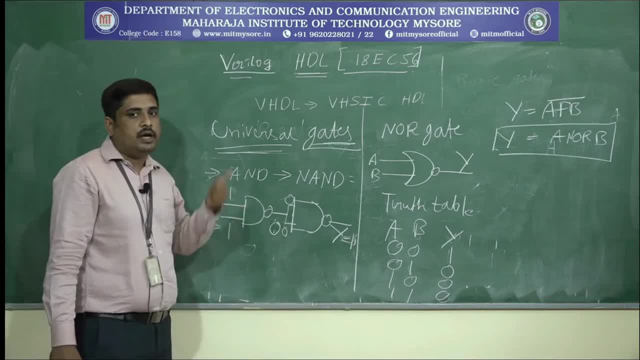 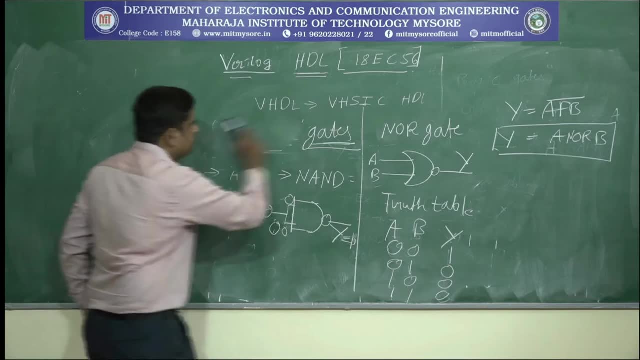 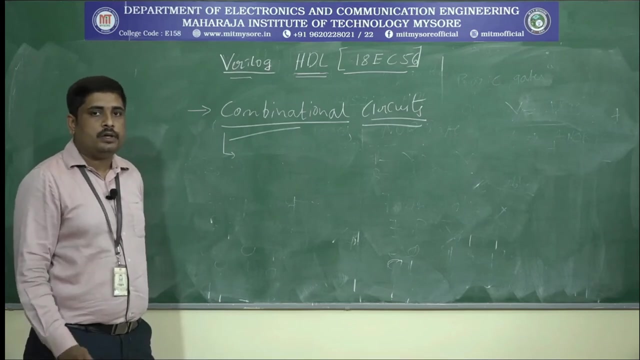 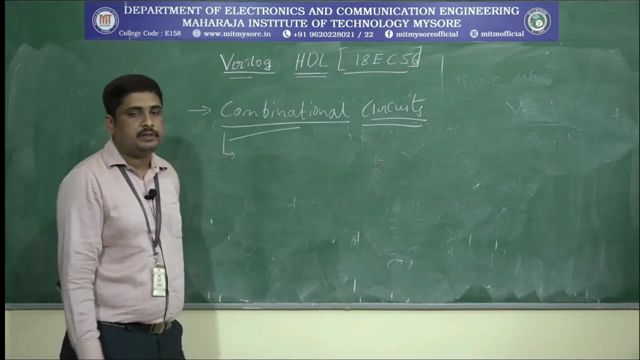 design. One is a we called as combinational circuits, another one is we called as sequential circuit. First we consider a combinational circuits. Combinational circuit- it is defined as the output- depends on only a present input. Again, I repeat: combinational circuit is defined as the output. 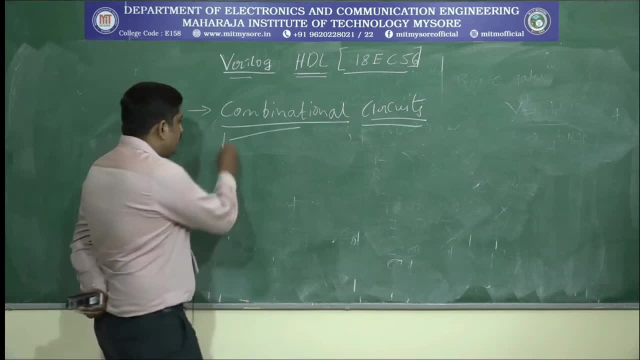 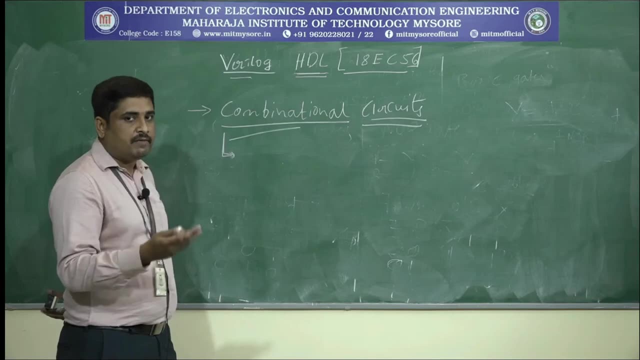 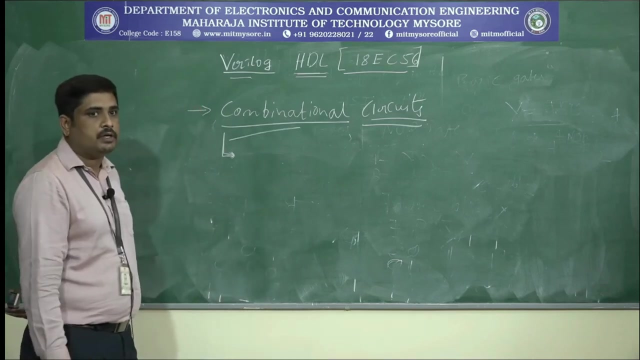 depends on the present input. So output depends on present input means any changes in input and that time the output changes quickly. So we called as combinational circuits Circuits. let us take some examples for combinational circuits. When you design the combinational, 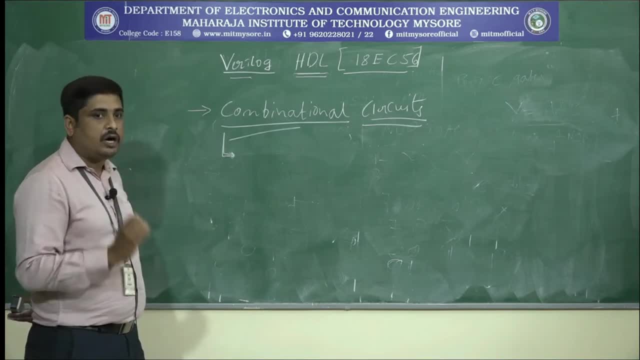 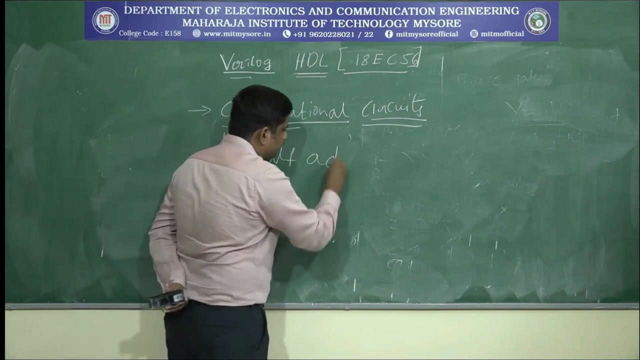 circuits. you should know the what all the gate operation is, because when you write any combinational circuit, the gate is what must and should gate is required. So combinational circuits, let us take basic circuits. basic one is off adder, off adder. 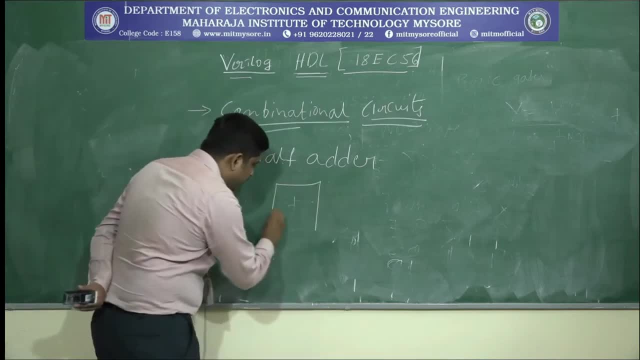 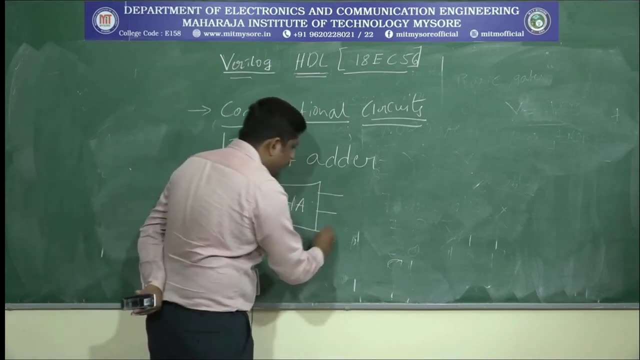 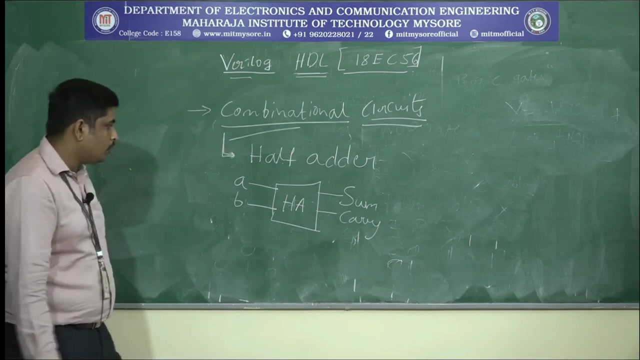 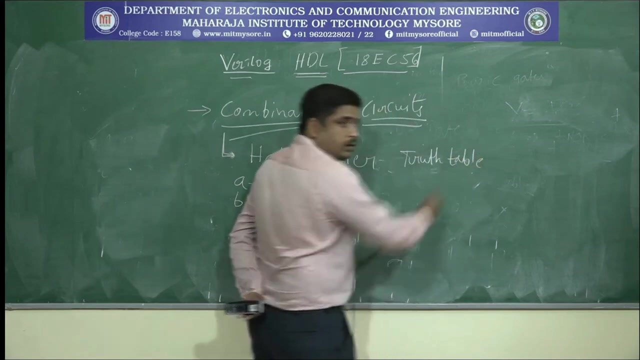 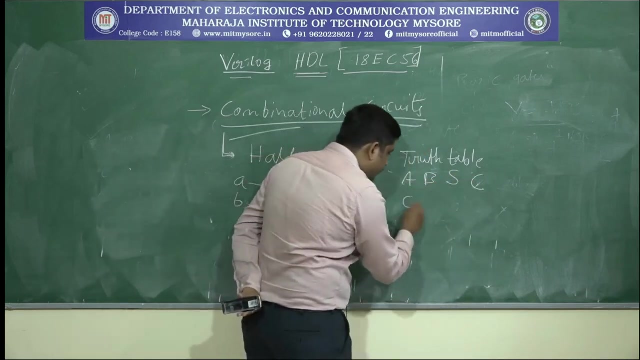 is the basic circuit. then we write the first back diagram for off adder A and B is the input, Two inputs here, Then sum and carry. Sum and carry is the output. First we write the true table. So true table A and B is the input, Then sum and carry is the output. So A and B when it is 0, 0. 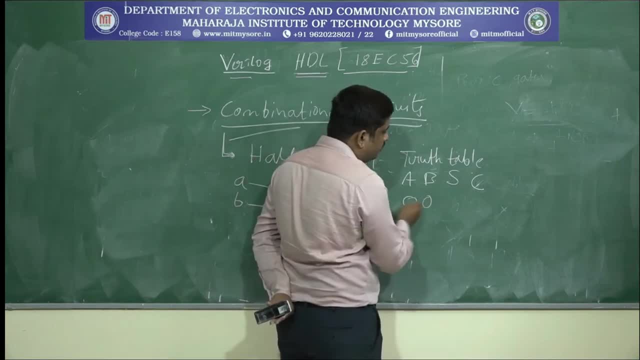 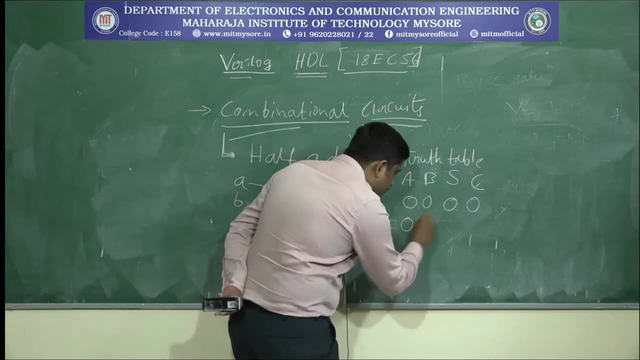 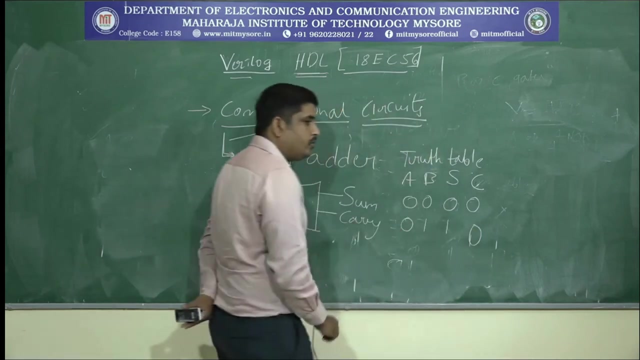 Then when you add these two, 0, 0, then sum is equal to 0, then carry is equal to 0.. When 0, 1 is the second combination, When you add 0, 1, then sum is equal to 1, then carry is equal to 0. 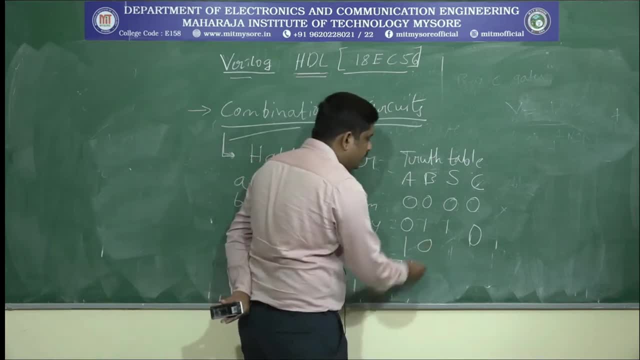 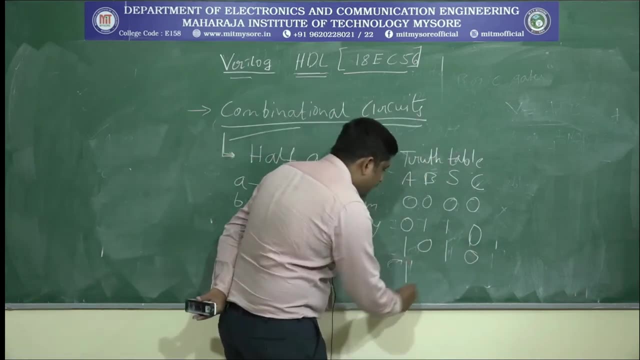 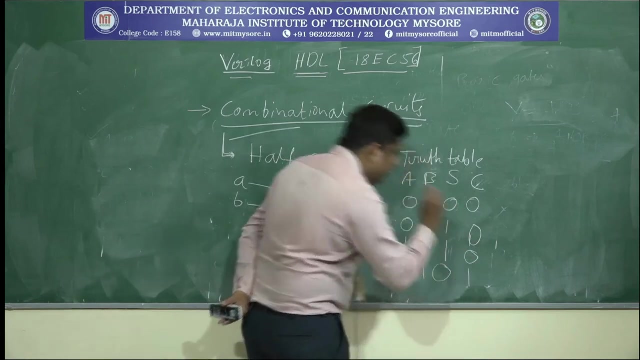 Next one: 1, 0.. 1, 0 you add, then sum is equal to 1, then carry is equal to 0.. Then last combination, B is equal to 1.. B is equal to 1, and that time add these two, then sum is equal to 0, but carry is generated. 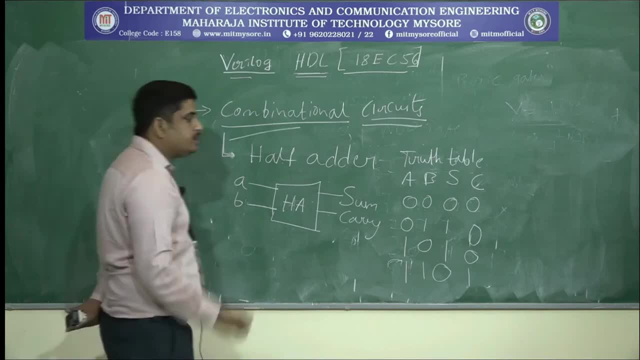 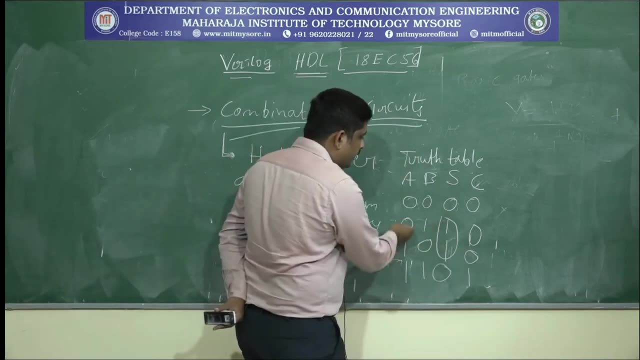 So this is the true table for a simple off adder. Based on this true table, we have to write the equations. So here, when these two condition, When it is 0, 1 and 1, 0, then the sum is I. 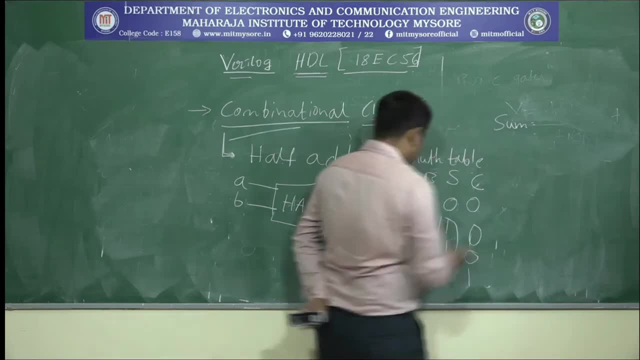 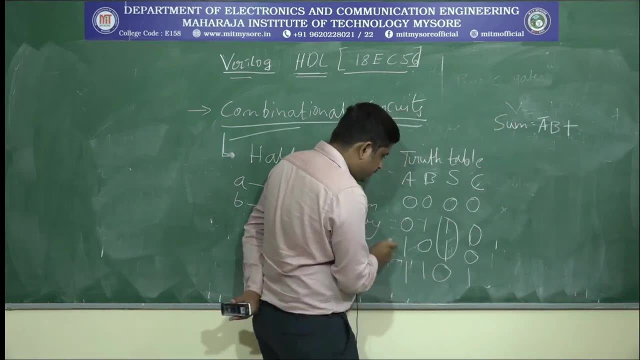 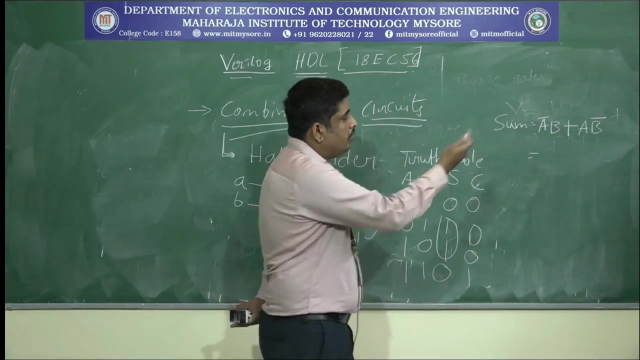 So it can be written as: sum is equal to: So here A bar B Plus next one A B bar. So you just observe the equations here. So it requires totally 5 gates 2, not gates, then 2 and gates 1 or gate. 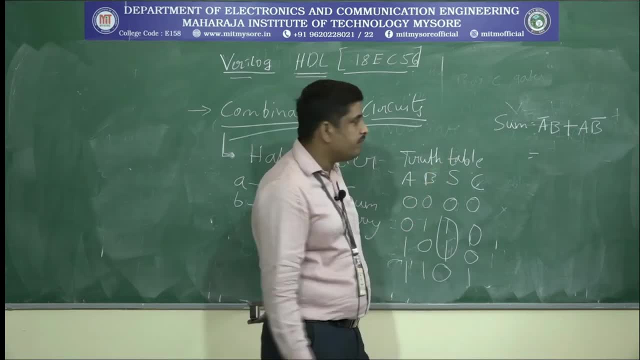 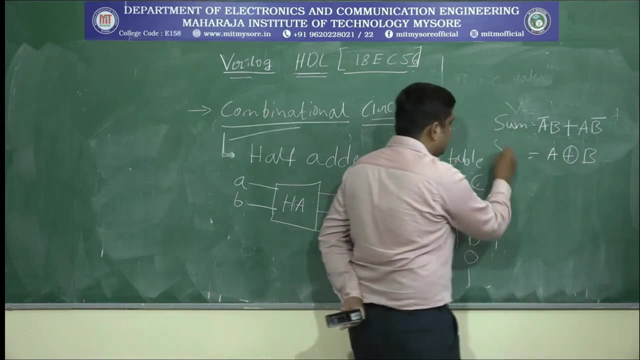 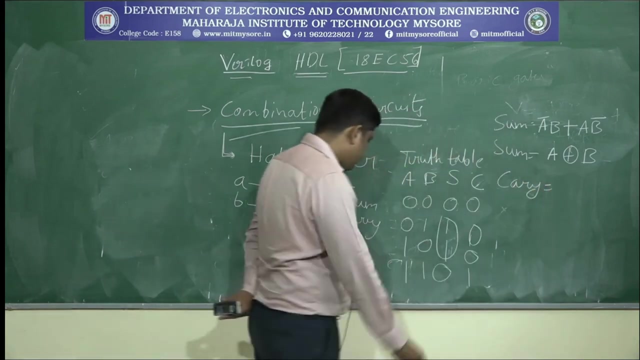 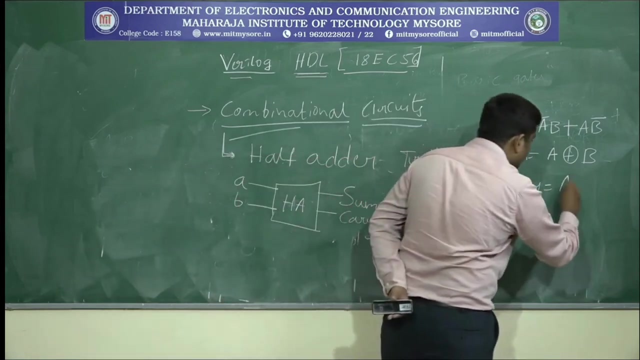 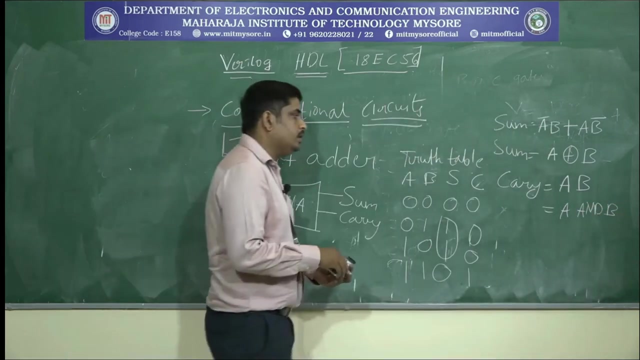 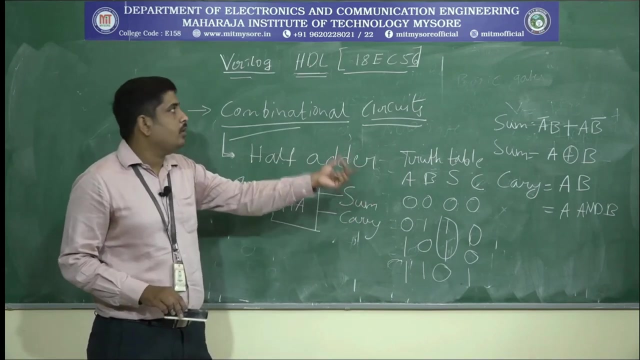 It is very difficult to implement. So that is why this equation can be modified So it look like a XOR gate, So it can be written as A XOR B. That is a sum equation We have to write. So if you write the carry equation, carry is equal to. just observe here: when it is carry is equal to 1. so that is last condition, that is A and B. so A and B or you can write A and B. this is the what, the final carry equations here. so using this equation, we have to write the, a programming language that is Verilog, HDL. 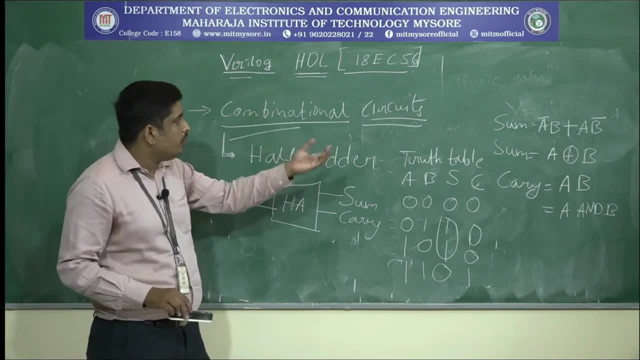 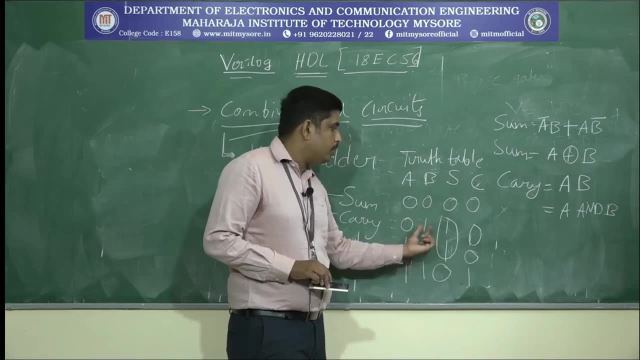 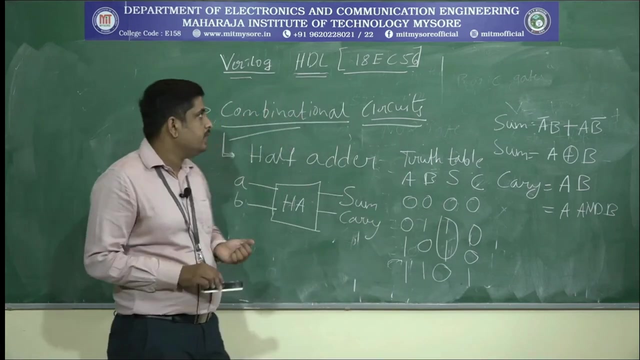 So this is the one example. So here we have to prove the output is directly proportional to what input. here, when it is 0, 0, 0, only when you changes the one input, that is, B is equal to 1, then output is changes quickly. that is, sum is equal to 1, then carry is equal to 0. 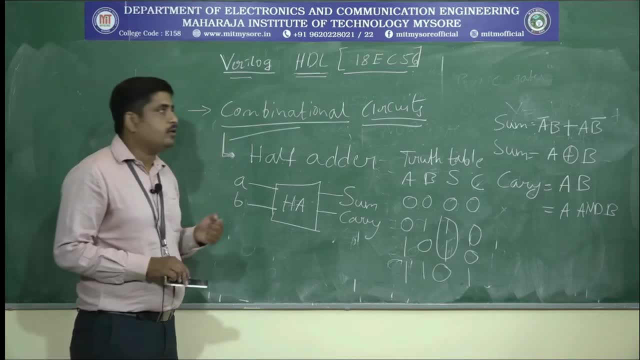 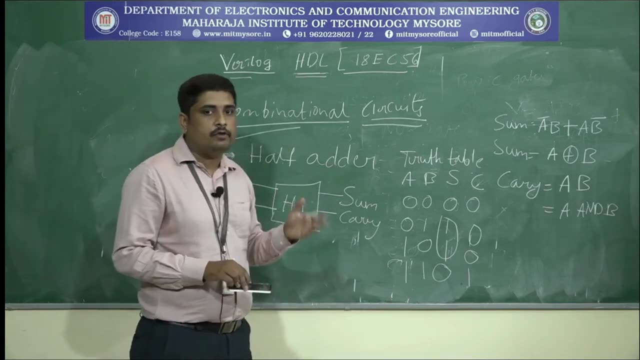 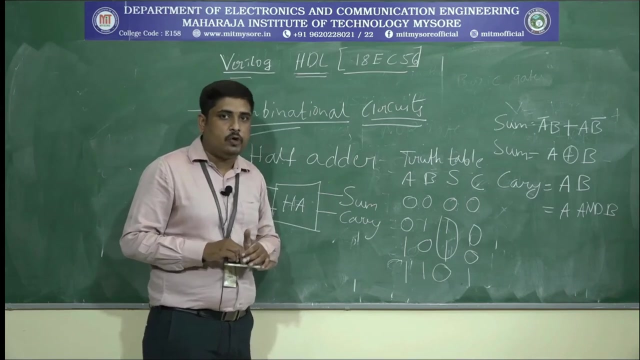 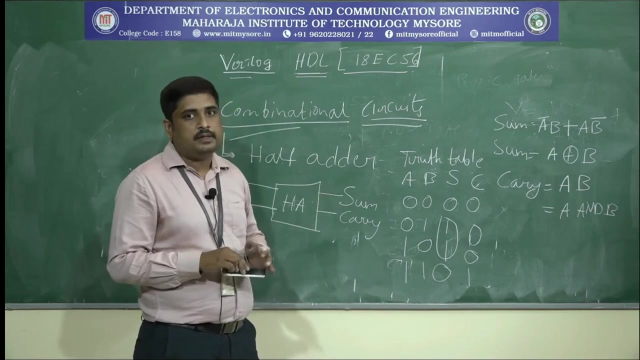 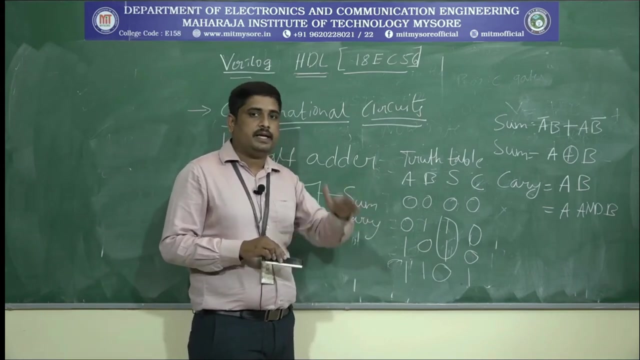 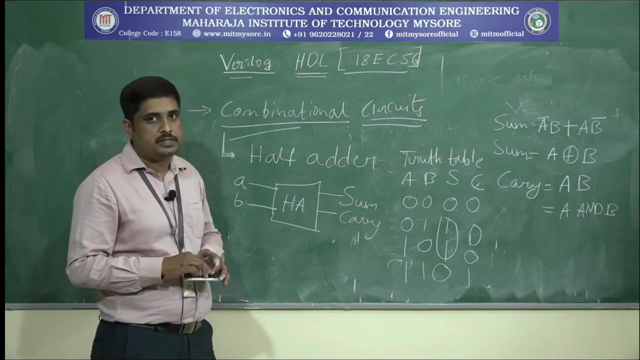 So many combinational circuits available with respect to digital system design: off adder, then off subtractor, then full adder, then full subtractors, then off. These are all the basic Adder circuits. and also there is a encoder. there is a decoder, then priority encoder, then without priority, then multiplexer, then we simply called as MUX. it stand for many into one, that is, many inputs then one outputs, then D-MUX. it's exactly opposite of a MUX. so many combinational circuits are available with respect to what a digital system design. 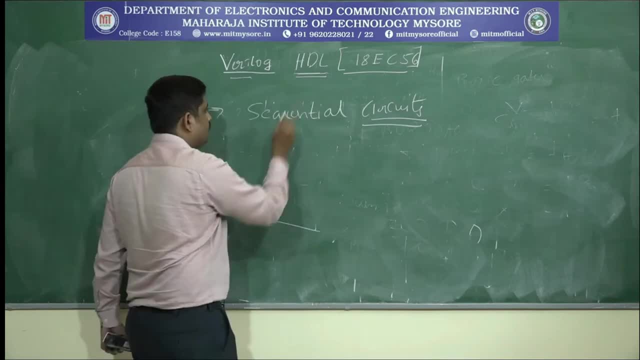 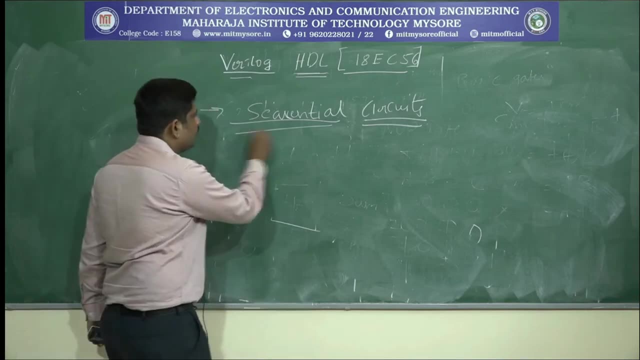 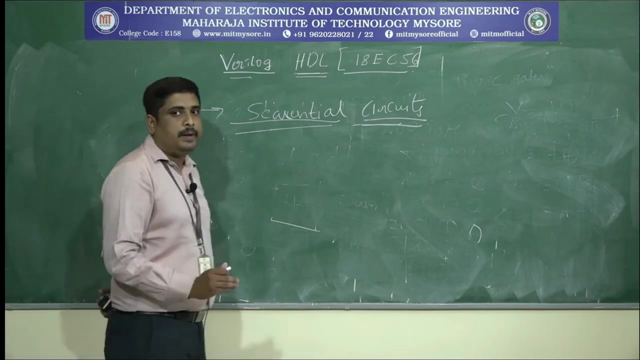 So next second one: sequential circuits. So it is defined as the output depends on the present as well as previous one previous input or it may be a output. again, I repeat this: the sequential circuits is defined as the output depends on present as well as past output. 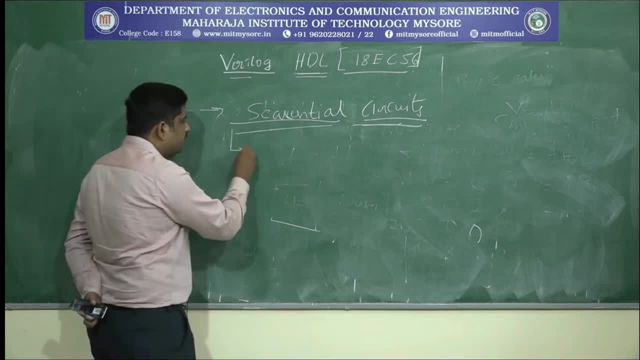 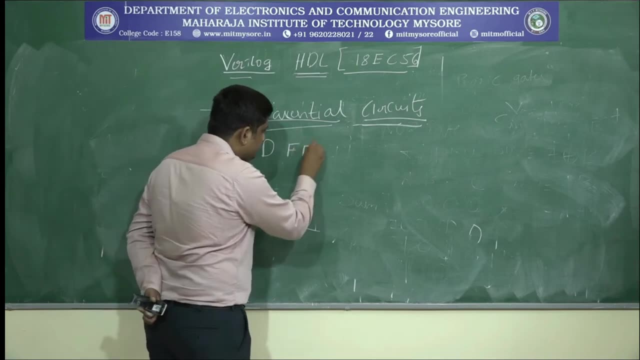 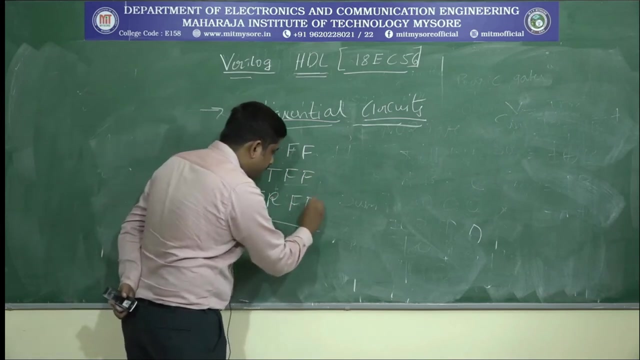 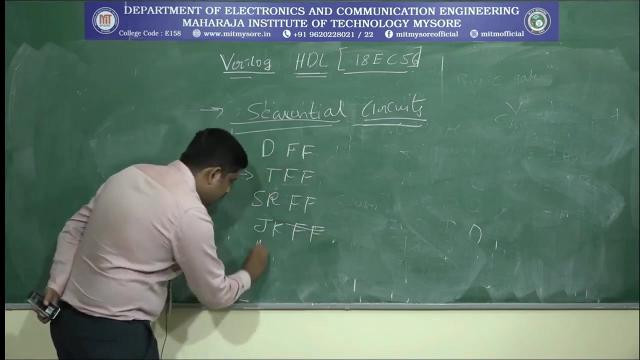 Or input. so here there are many sequential circuits. here we start, go with what a flip-flops. so first one is the basic one: D-flip-flop, then T-flip-flop, SR-flip-flop, then JK-flip-flop, MH-JK. 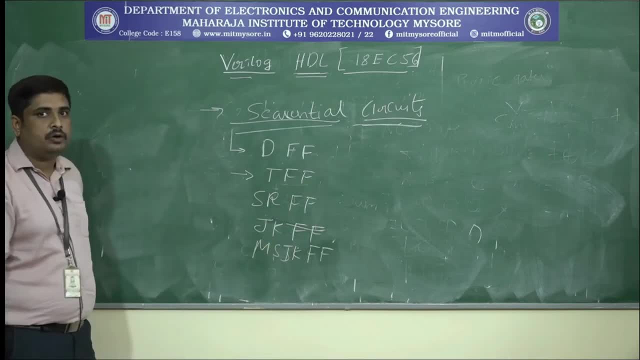 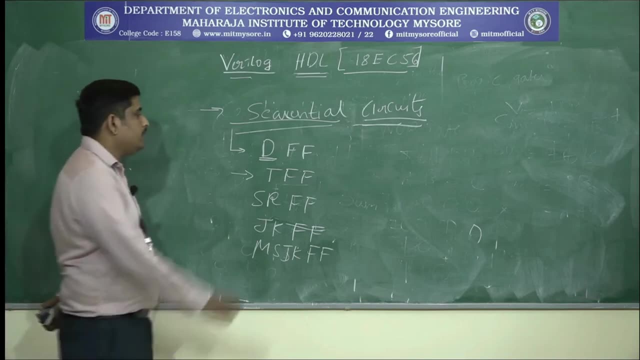 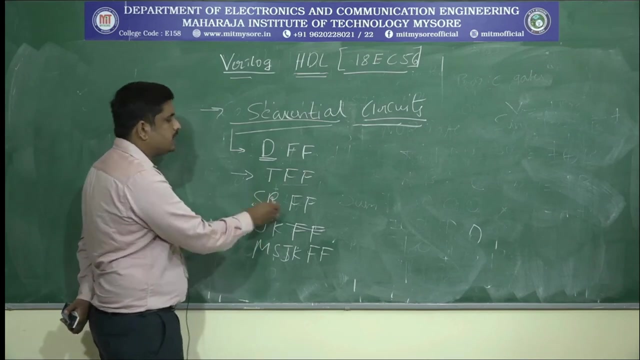 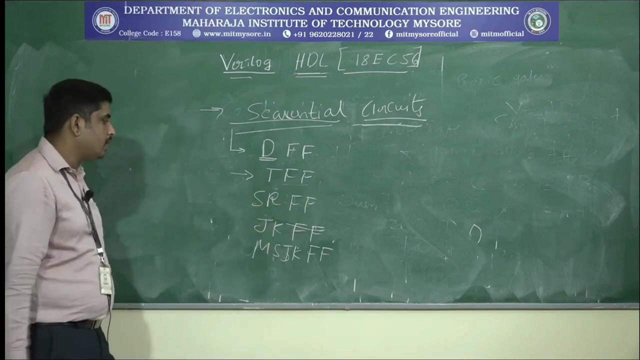 Flip-flops. so these five flip-flops are available with respect to sequential circuits. so here D-flip-flop, the D indicates its delay or data. flip-flop, then T-flip-flop, we called as it's a toggle flip-flop, then set or reset, or we called as SR and RS. okay, then set, reset flip-flop, then JK-flip-flop, that is J and means Jack and Kilby, the scientist name JK-flip-flop, then MH-JK flip-flop. 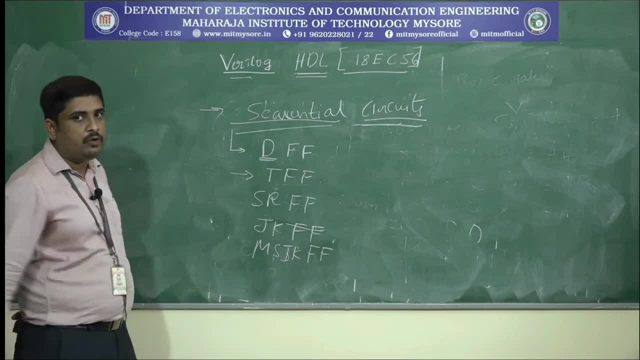 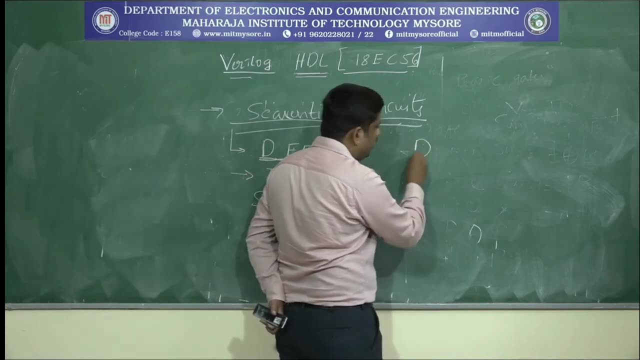 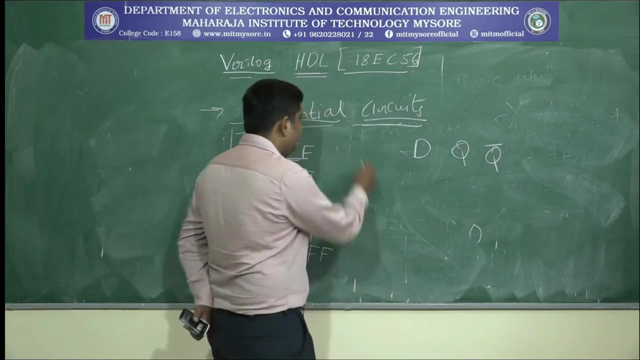 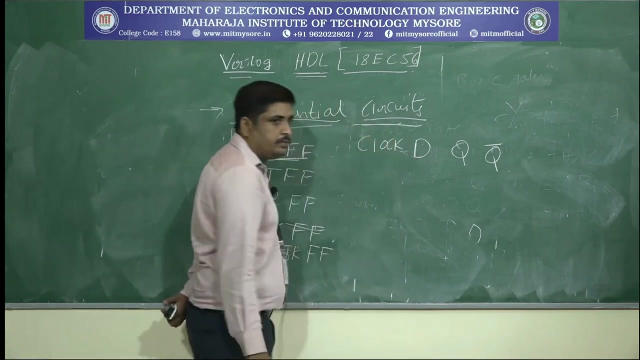 So let us consider one example. okay, with respect to sequential circuit, we simply: we take a D-flip-flop, we write the D-flip-flop root table, then D, then Q, then, if you want to complement this one, we write Q-bar. then obviously it's a sequential circuits. we have to assume the a clock pulse. okay, then either you can assume edge trigger or level 2.. 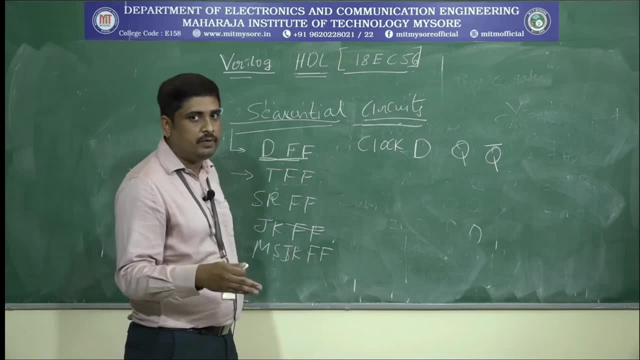 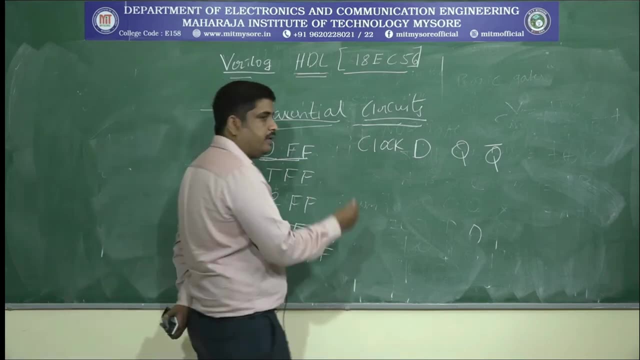 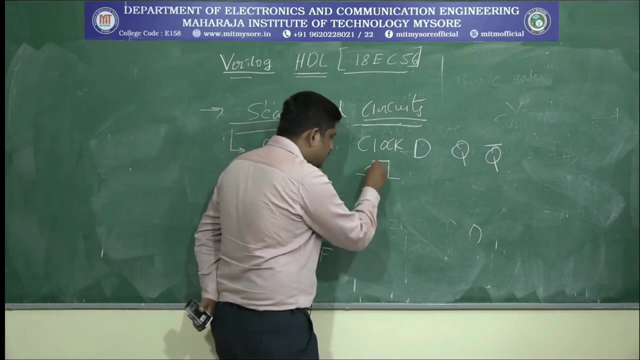 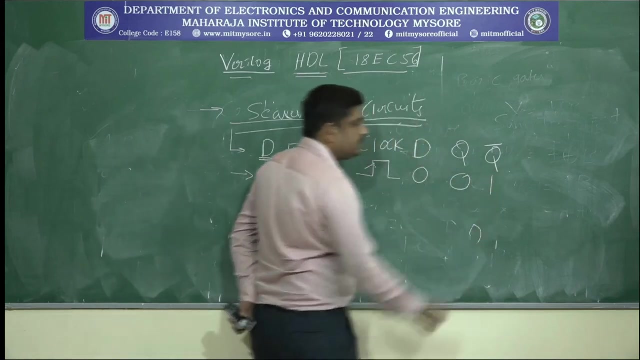 So we always choose edge triggered flip-flop because it changes a quickly, but level triggering is the speed is very less okay. so that's why we always choose edge triggering. that is, either you assume positive edge triggering or negative edge triggering. So let us assume positive edge triggering. when D is equal to 0, then Q is equal to 0, then Q-bar is complement, it's 1, then again one more clock you applied, that is. 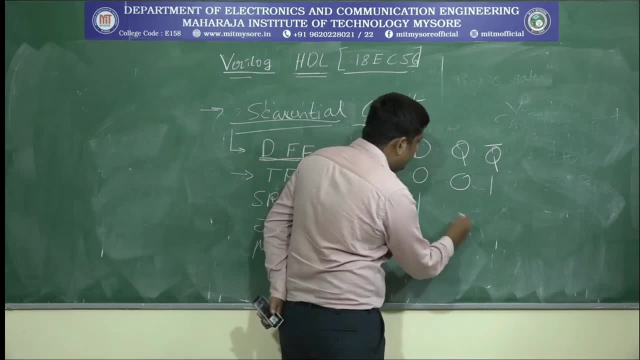 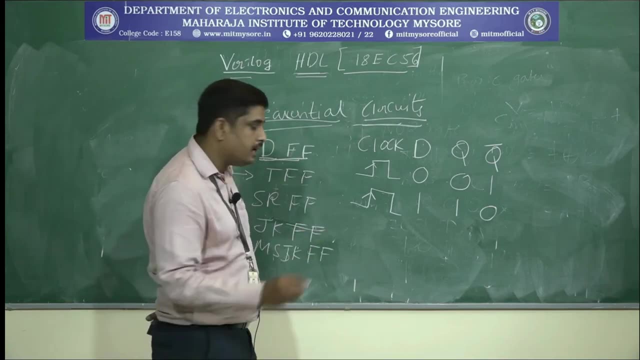 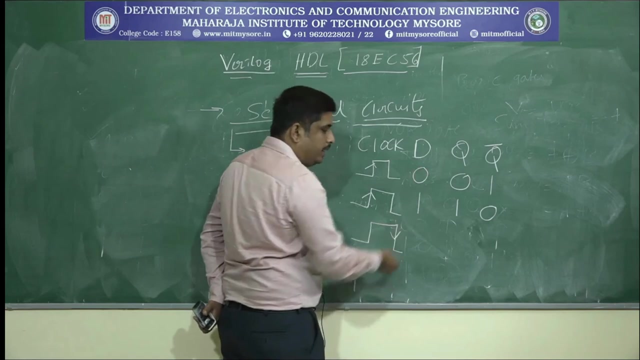 Positive clock pulse again when it is 1, then here Q is equal to 1, then Q-bar is equal to 0.. So this is the what: when you applied the positive edge triggering, so when you applied the negative edge triggering, what happens here? when you applied negative edge triggering, so here D, either 0 or 1, okay, we called as a, simply don't care, either 0, 1 you applied. then whatever the previous one, that is, previous state, is repeat. here that is 1.. 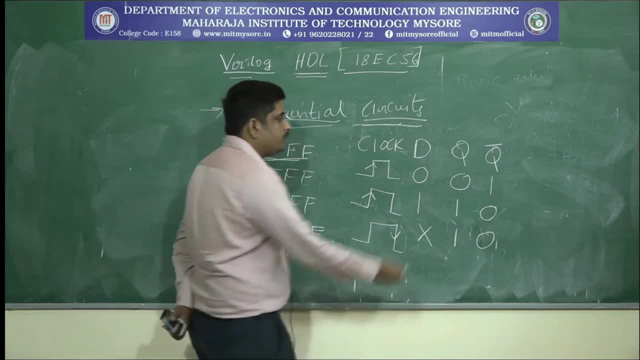 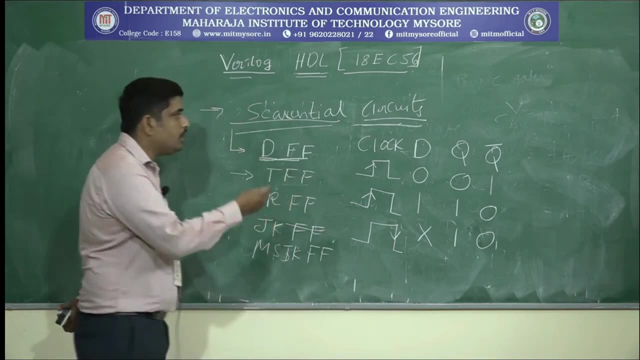 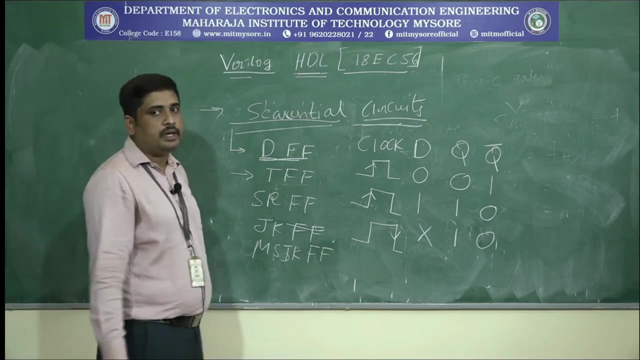 And 0. okay, so that is previous. state is 1 and 0, so it follows the previous state, that is 1 and 0. so this is the what example for sequential circuits. so not only flip-flops, there is more sequential circuits. so counter is there, then shift resistor is there. so these are all the what the basic needs for a Verilog HDL. 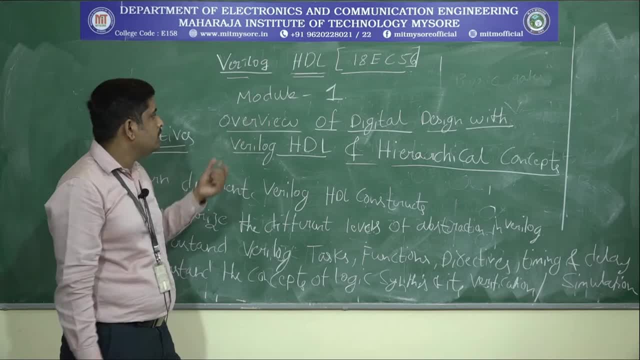 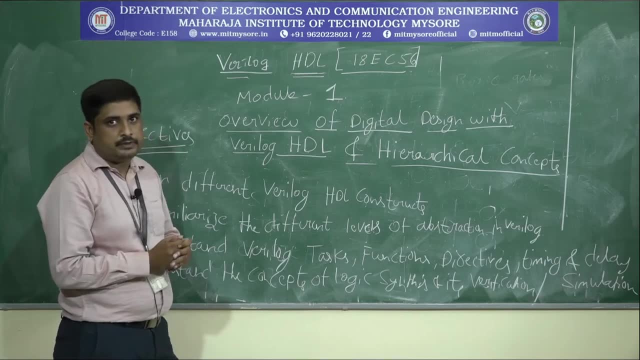 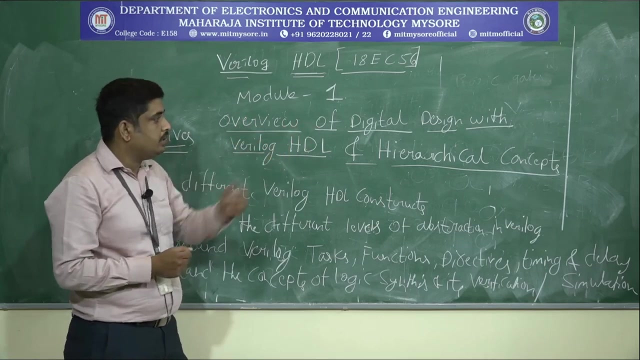 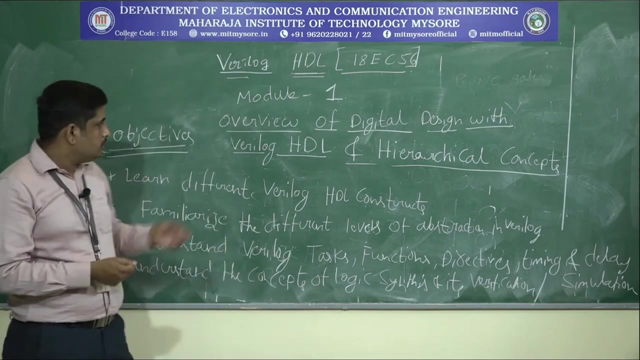 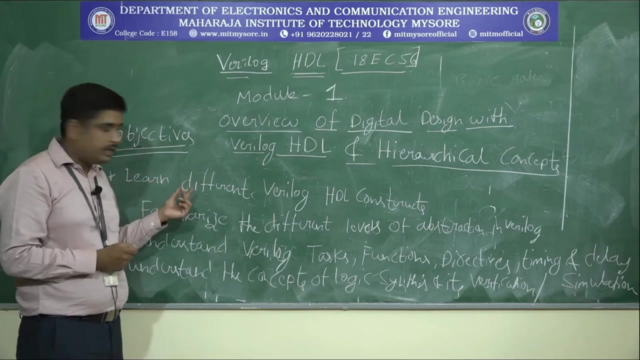 So next, module 1, the name of the modules, overview Of digital digital design with Verilog HDL and hierarchical concepts. so here there are two parts here: overview of digital design with Verilog HDL. it's the first part, then second part, then hierarchical concepts. so before going to module 1, first what are the objectives regarding a throughout the subjects? the first objective then: learn different Verilog HDL. 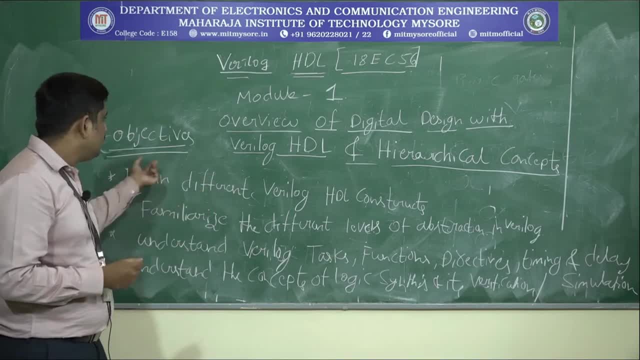 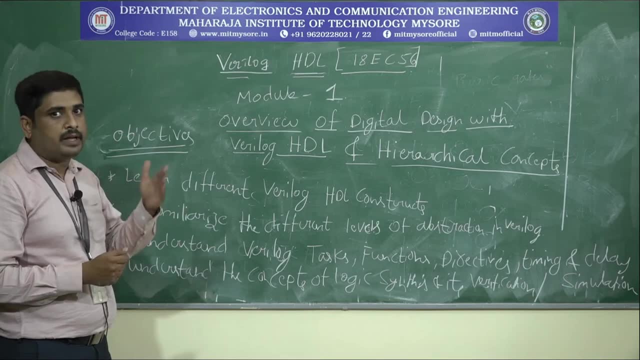 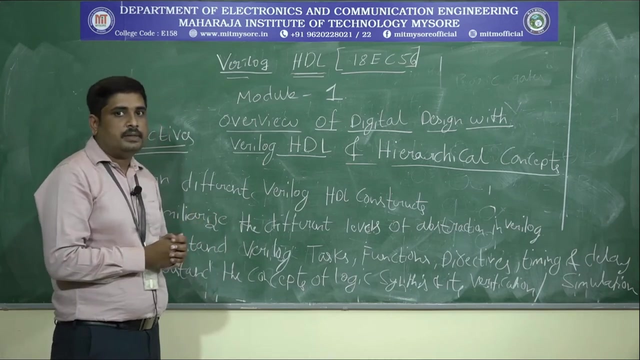 So here the first objective. it's related with module 1 and first of the module 2, that is part a for the module 2, the HDL constructs, in the sense we have to discuss some basics of HDL, then hierarchical concepts and some programs related. okay, so that is comes under, then HDL constructs. then 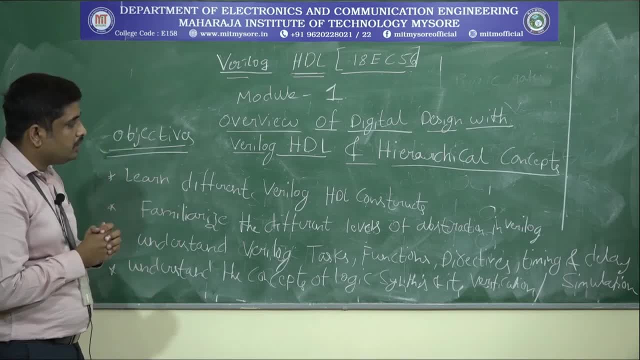 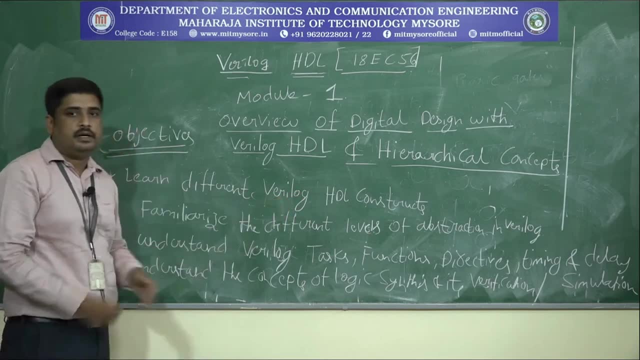 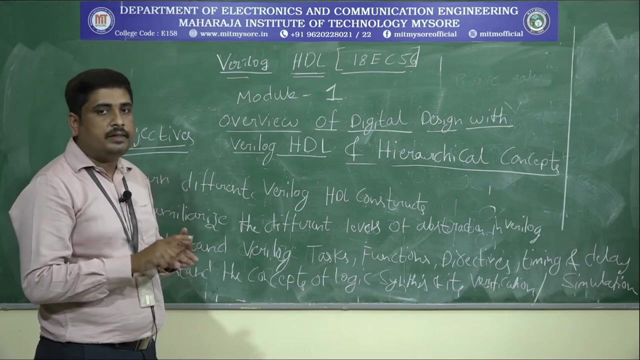 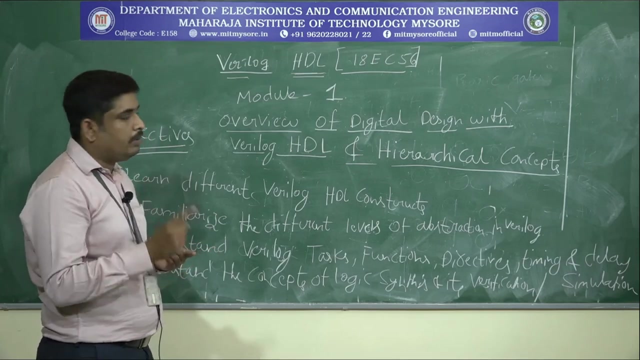 Second one familiarize the different level of abstraction in Verilog, so usually the Verilog abstraction in the sense. then three level obstructions we have to consider here: then data flow, gate level, then behavioral. so in the gate level it is module 2, then the module 2 second part, then remaining one that is a behavioral and data flow. 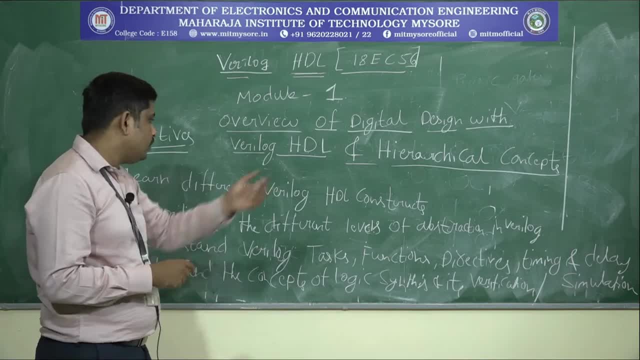 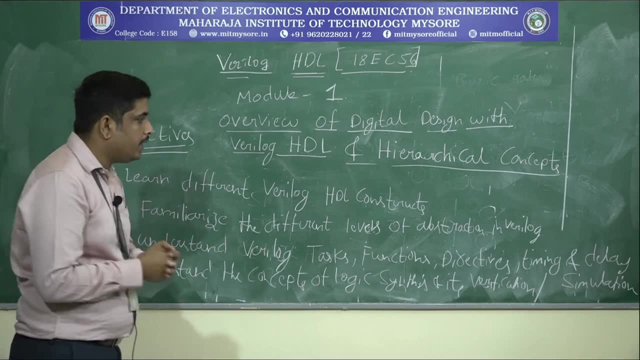 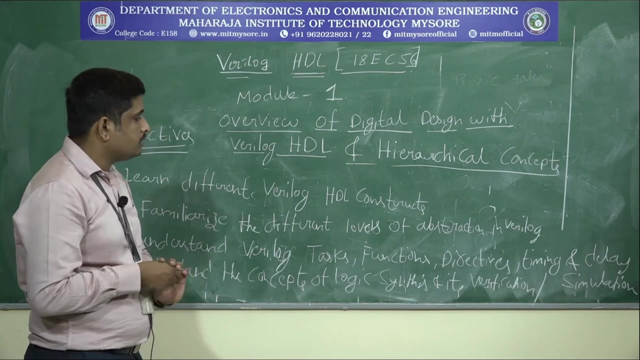 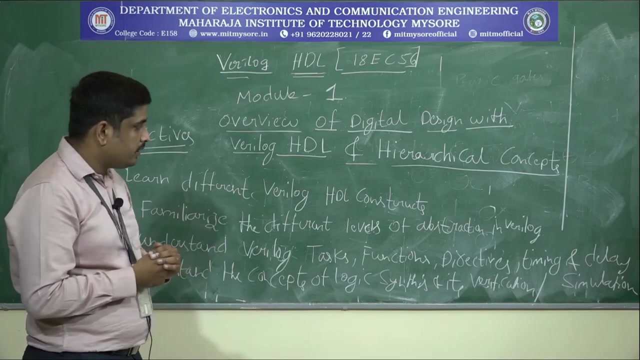 So that covers a module 3. so that is the what is second objective. then next objective: understand Verilog tasks and functions, directives, then timing and delay simulations. so here we discuss tasks, then functions, then what's the difference between tasks and functions then with respect to directives? we have to discuss then after this, directives. 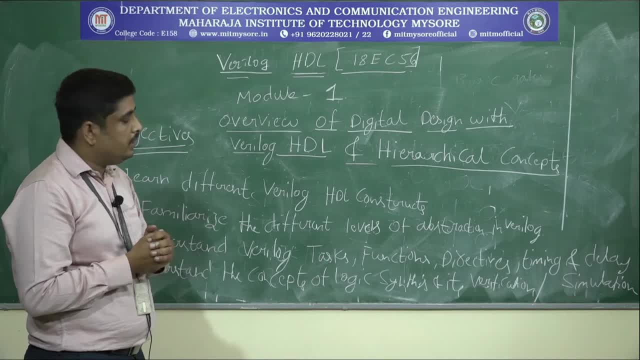 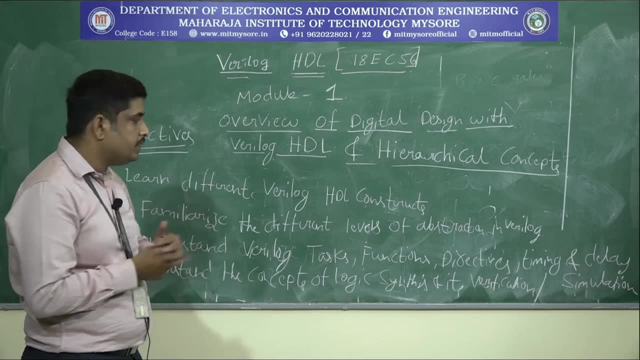 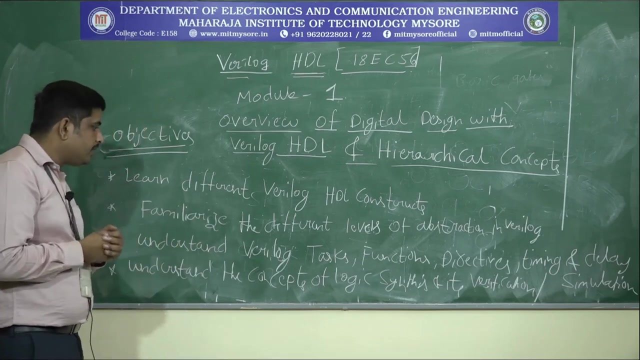 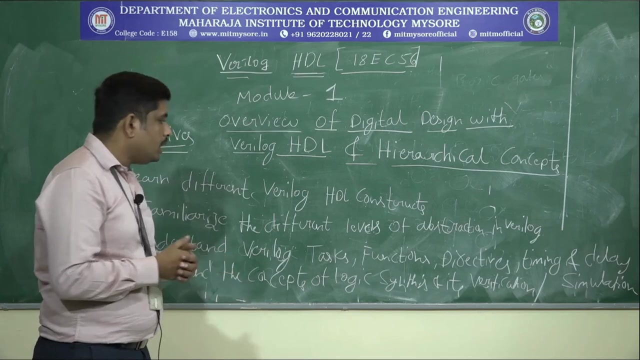 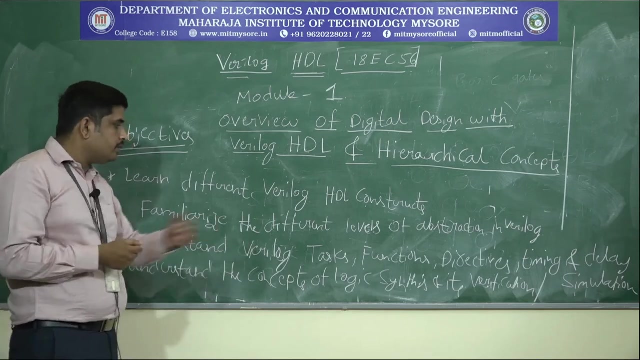 Then Directives, Directives, Directives, Directives, Directives. Then we calculate the timing, then as well as delay with respect to simulations. so it comes under that is. this objective covers module 4. then, last one, understand the concept of logic synthesis and its verification. then this one- it's introduced here for new syllabus 18 scheme. so understand the concepts of logic synthesis. 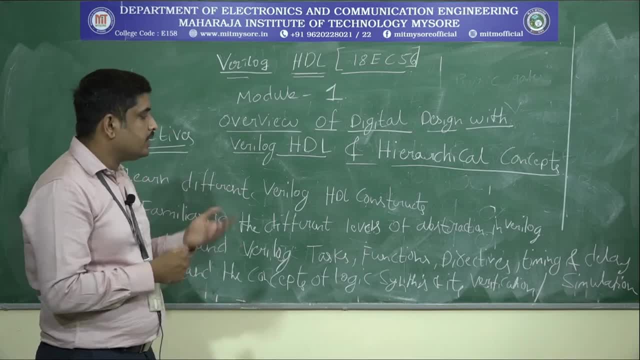 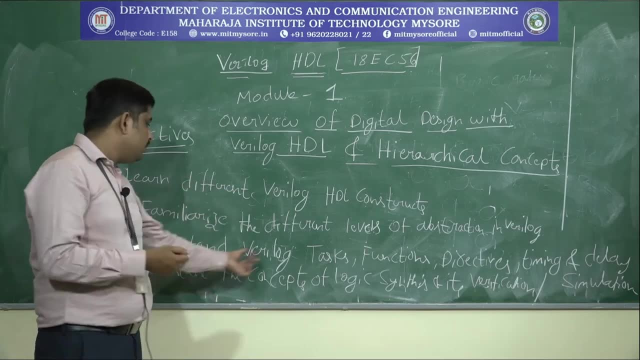 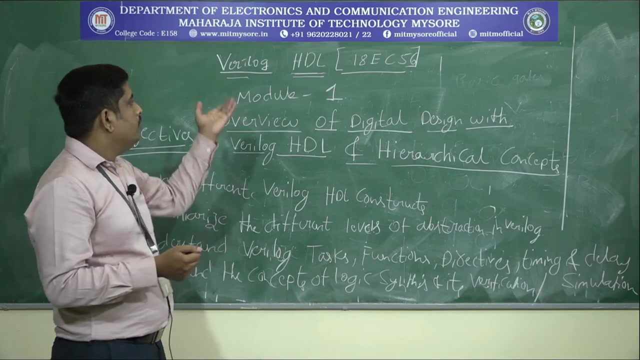 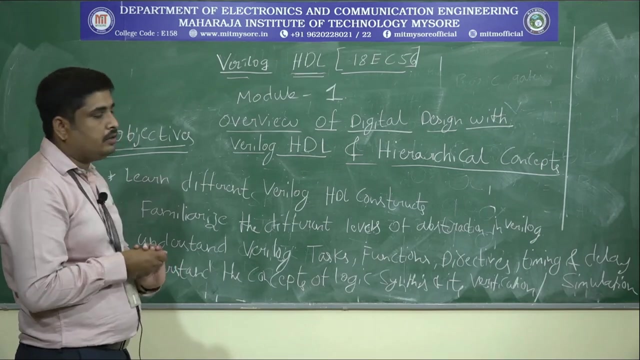 Logic, synthesis and verification. synthesize the circuit as well as verification done in what. that is objective. so it this for objective. that is fourth objectives. it's related to module 5, so again first want to consider module 1, overview of digital design, Verilog, HDL and hierarchical concepts. so in module 1 first, 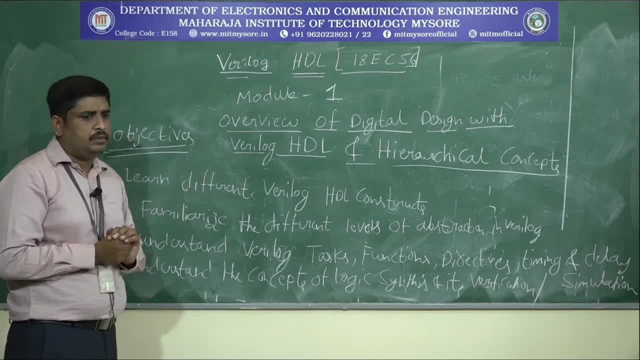 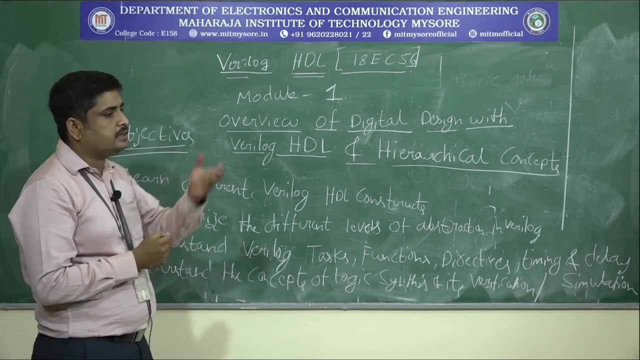 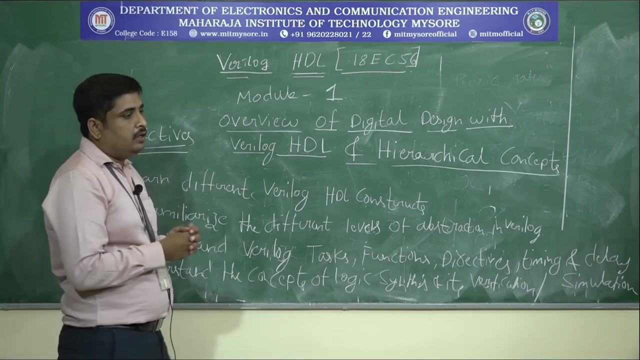 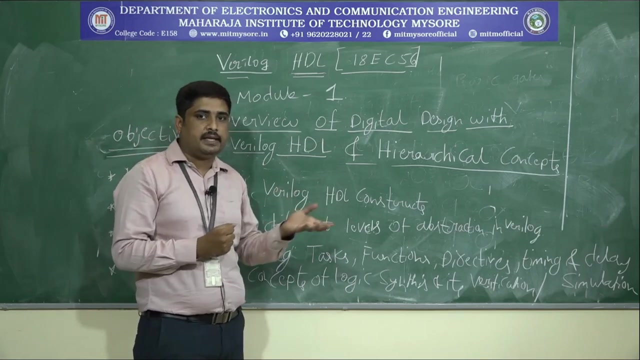 With This We discuss about evolution of CAD, that is, CAD is what it's very popular word, computer aided design. so we discuss just history of the CAD. then next one: it's related to subject that is, emergence of HDL. so why HDL is required, why not HDL? so two concepts: it covers emergence of HDL. next, typical HDL design flow. so how to design a ICL. 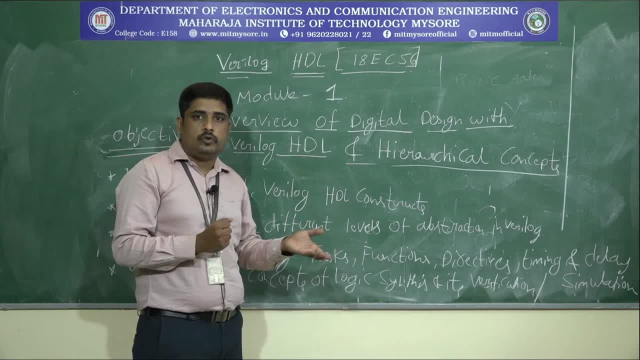 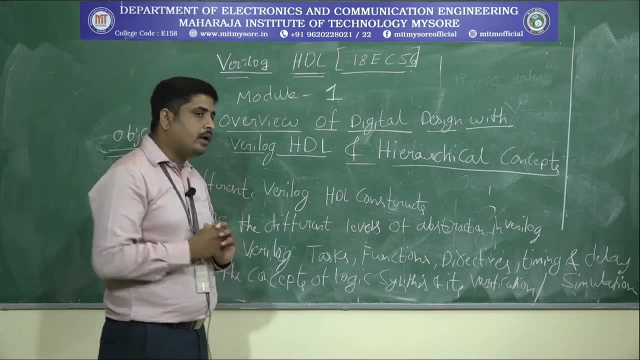 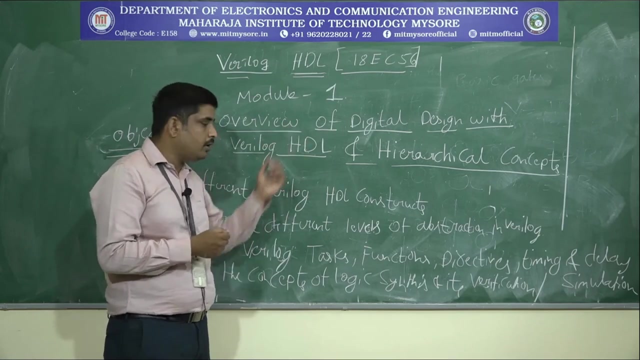 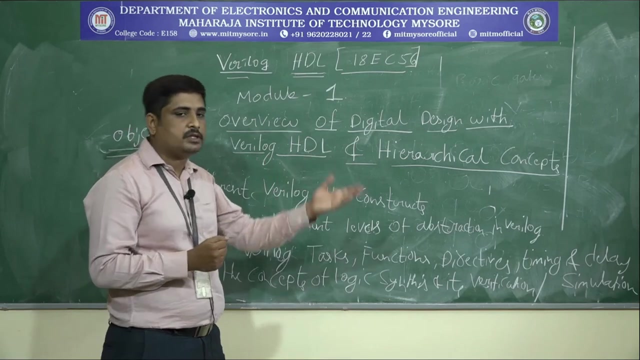 Using HDL, and as well as one more tool is there, that is, we called as EDA, electronics design automation tool. then, after this, what are the importance of HDL we discuss? then, last one of the what a part. this part is a: why Verilog HDL? why Verilog HDL? in the sense we just compare that Verilog HDL with respect to another one, VHDL. so that is why Verilog HDL. then part B is: 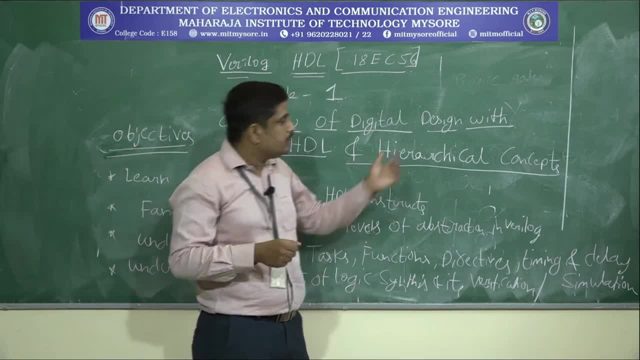 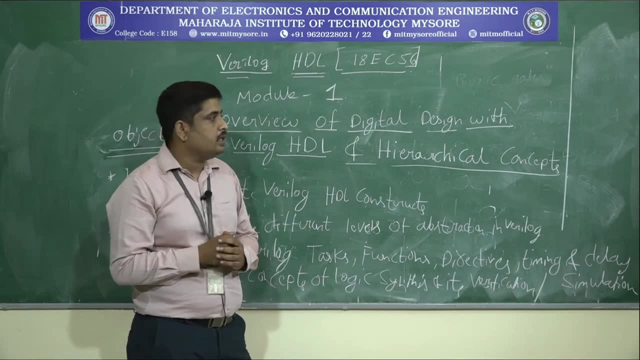 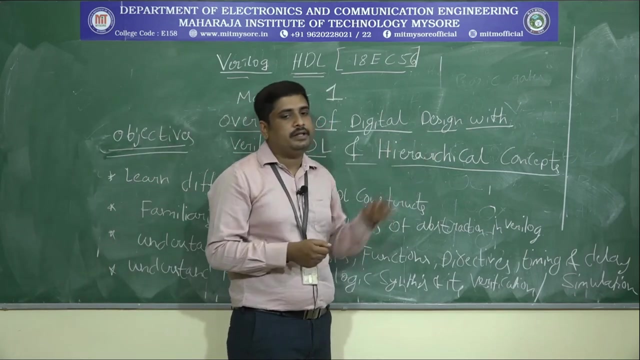 What I recall, concepts. so in I recall concepts of the name indicates here. there are two hierarchy here. one is a top down approach, another one is bottom up approach. we have to discuss, so we have to write the examples for both top down and bottom up approach. it comes under what I recall, concepts. so this is the what. it's just a overview of a module one, the first. 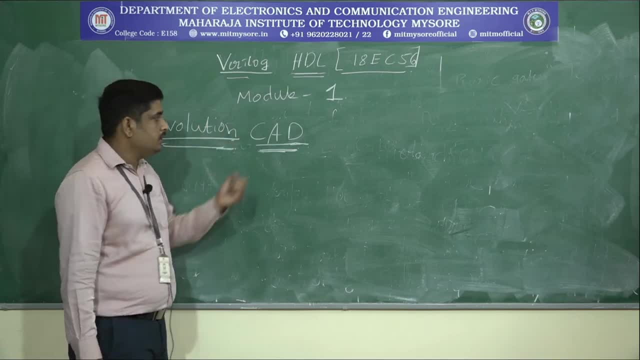 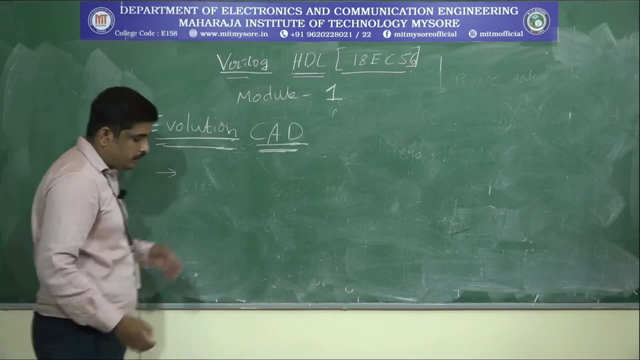 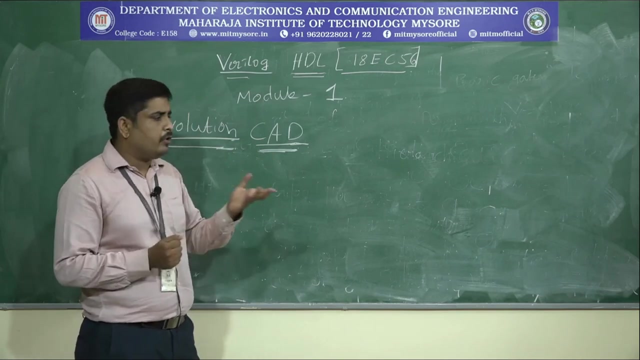 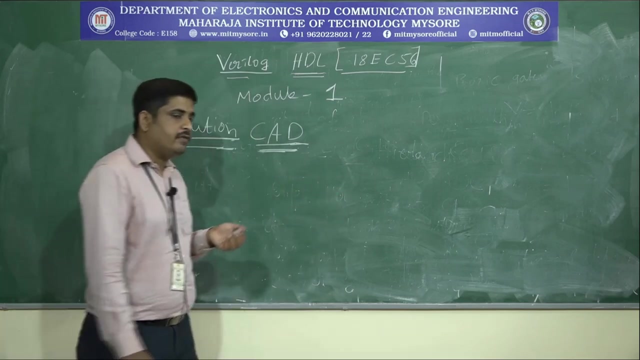 Topic of the first model is evolution of CAD. so the CAD is very popular word, that is, computer aided design. here, when you using the HDL language, we concentrate on only a digital circuit. we can possible to apply analog circuit as well as a mixed both analog and digital circuit here. from past 25 years the digital system design is rapidly developed. 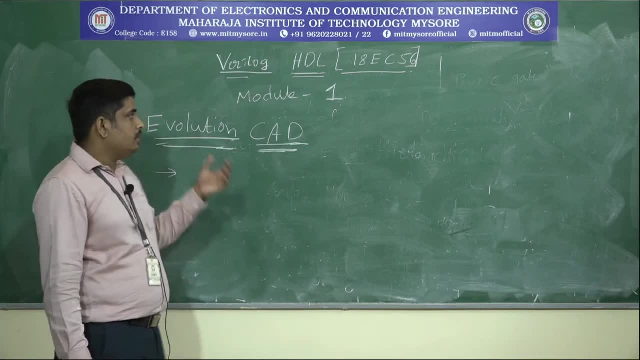 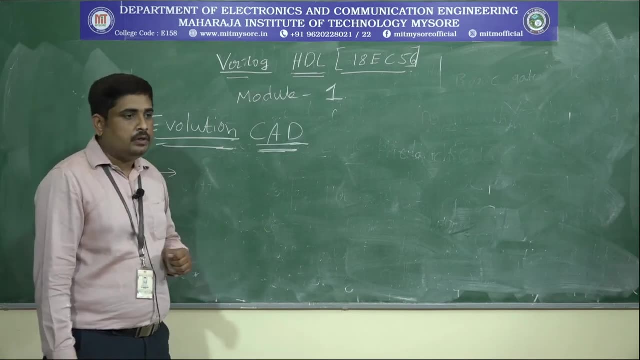 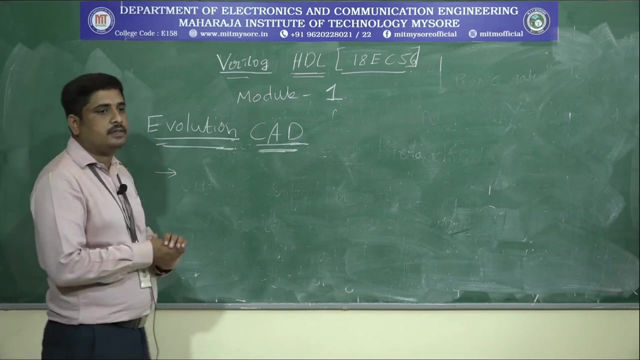 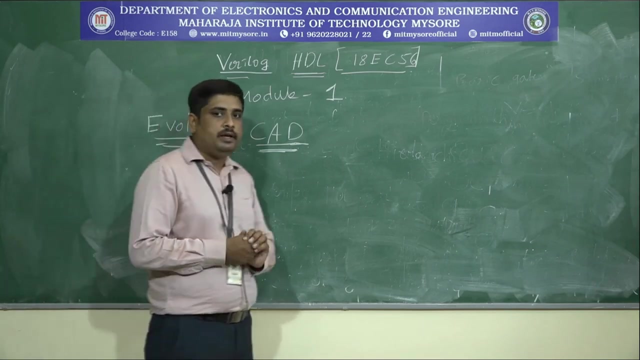 So in earliest, in earliest, the digital circuits or digital system design done with transistor and vacuum tubes. so the vacuum tubes is the what, the first generation of the electronic circuits. so next a transistor, so transistor, invented in 1947 at Bell Laboratories by William Shockley and his team. but there is a disadvantage. 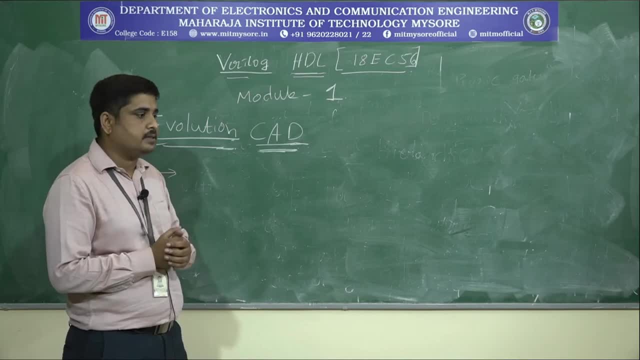 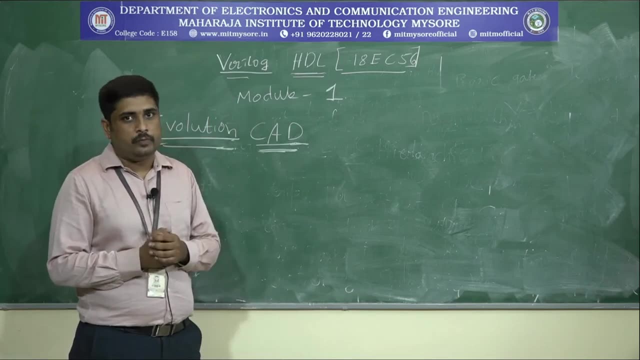 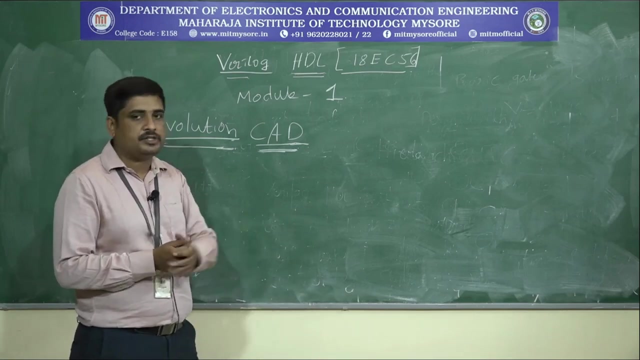 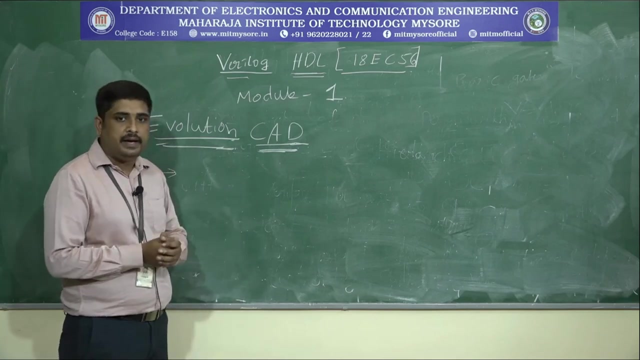 In Both vacuum tubes and transistors. so what are the disadvantages? let us take a vacuum tubes first. so just observe the what world radio. okay, the size is what. it's very big. but you just compared to 2010 or 2000, this generation radio. it's very compact. it's the size is what, it's very less. so that can happen using a integrated circuit. 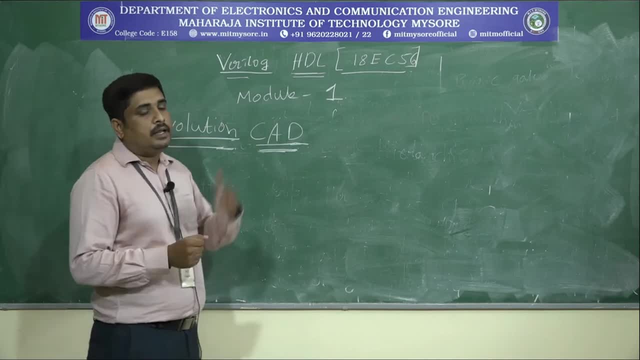 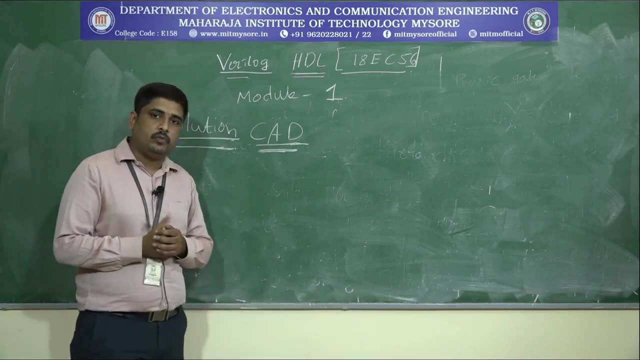 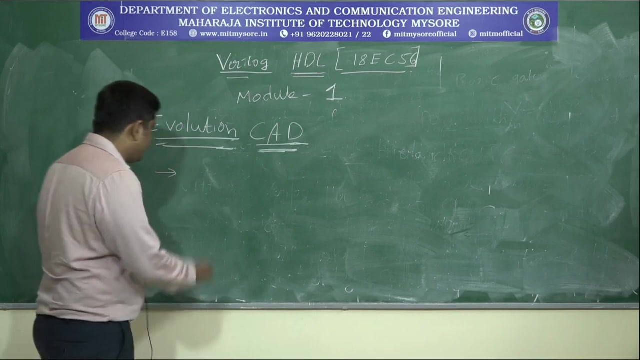 Transistor is. also there is a disadvantage because in earlier transistor it Come Consumes more power, usually 5 to 10 volts, but today's transistor, the it starts with what? 1.2 volts. so these two are disadvantages. it overcome by using the popular word, that is, IC. we called as integrated circuits. The first IC was officially generated in the year of 1960. then after 1960, the Transistor, that is IC generation, is developed rapidly. okay, the first IC is officially announced 1960. then after this, in terms of a generations, okay, the first generation IC we called as: 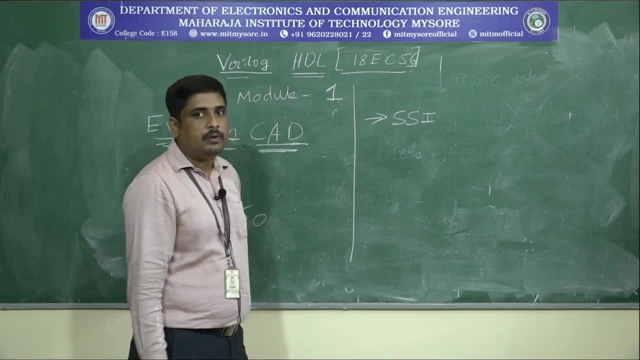 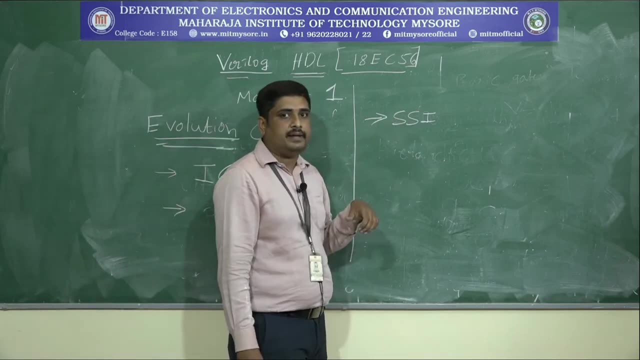 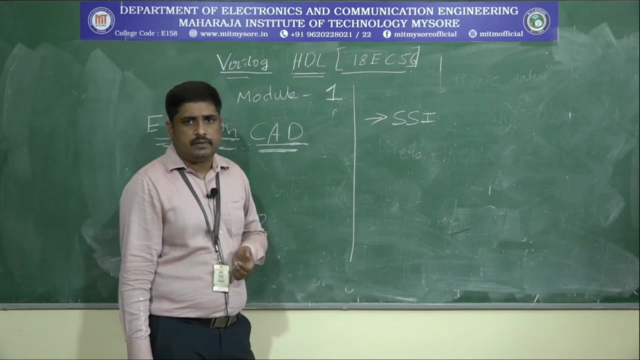 SSI, the name. it stands for small scale integration. the name indicates here in SSI, very less number of transistors, the very few number of Transistors, the very few number of Transistors. best example for this we have to consider a basic ICs that is 7404, then 7400 NAND gate. so these are all the what examples for small scale integration we called as a first generation. 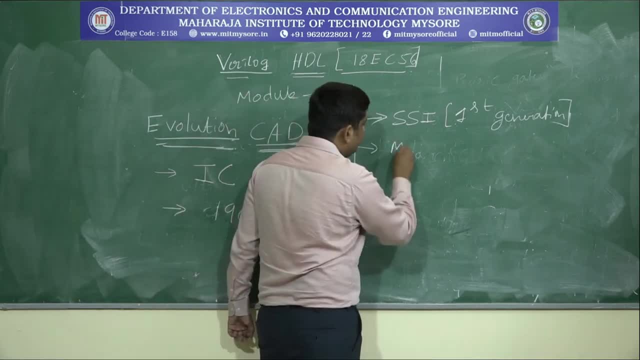 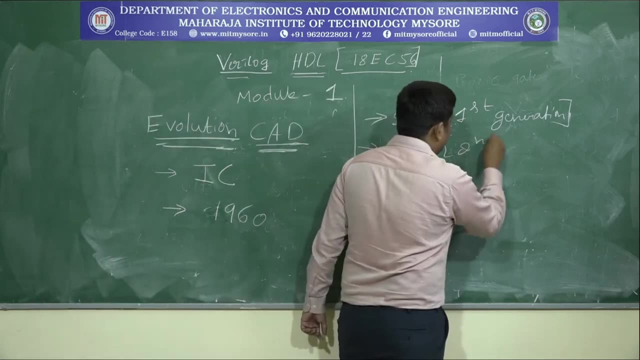 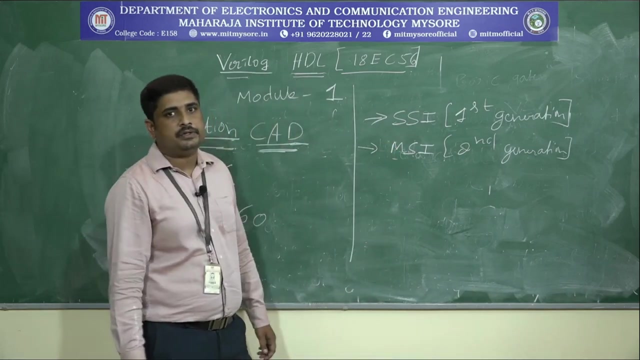 IC. okay then, coming to second generation MSI, that is, medium scale integration. so this one we called as a second Generation IC. so the name indicates medium scale integration. so here the unread number of transistors, or sometimes some books, is given thousand number of. 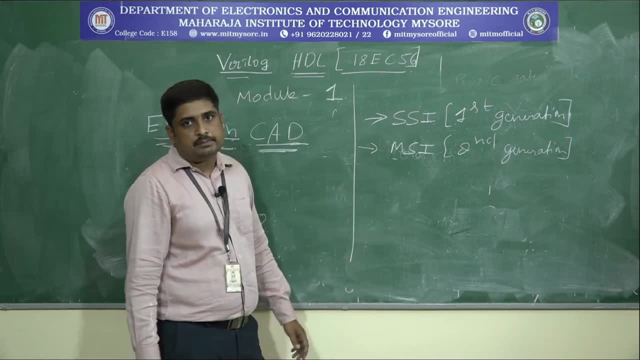 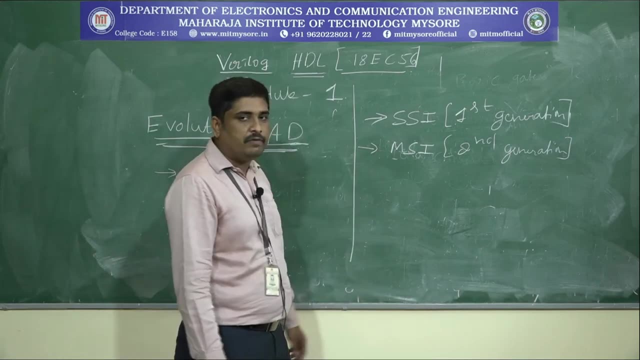 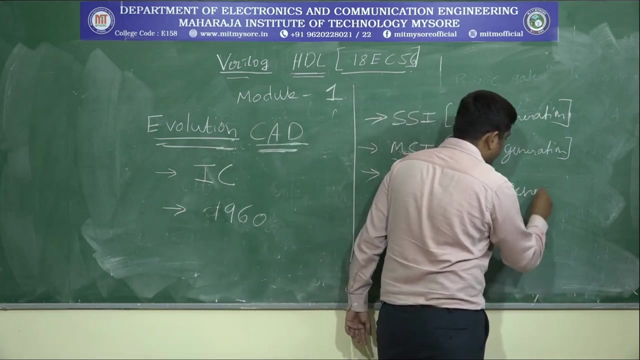 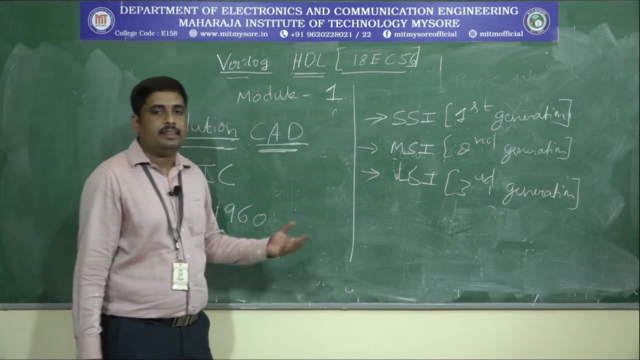 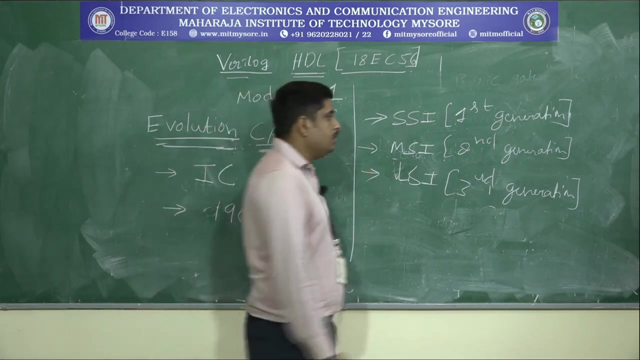 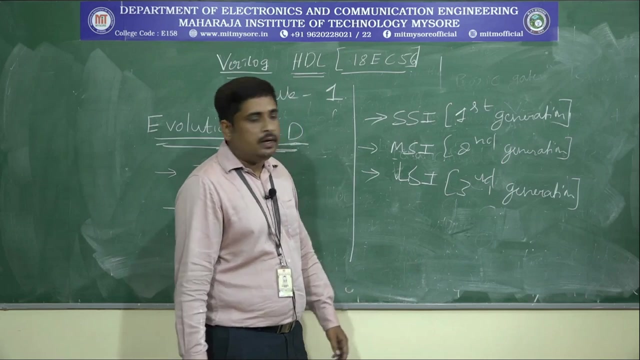 Transistor in a single IC. so best example for MSI is encoders, decoders, multiplexer and demultiplexer. this is the example for MSI. next LSI. So in a LSI it's a thousand number of or ten thousand number of transistor in a single chip or a single ICs. so here earlier microprocessors, so we name it as 8086, 80186, these are all the earlier microprocessor is done with with respect to third generation IC, that is LSI. then next one, which is very popular one,